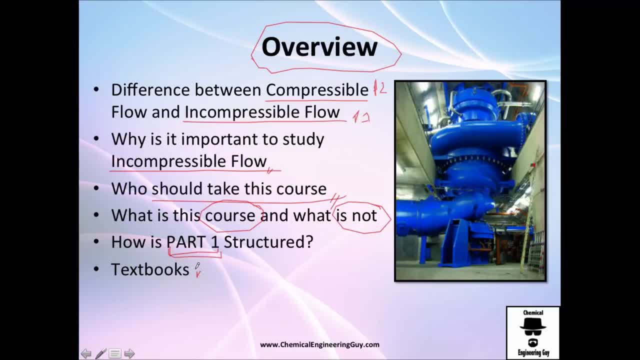 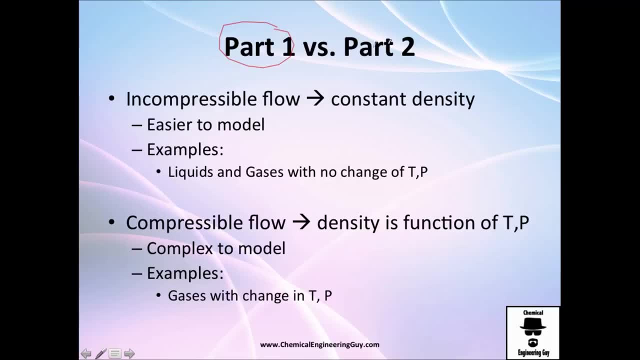 incompressible flow is structured And finally, we check some textbooks. So first things first. let's see why I choose to split part number one and part number two. Essentially because part number one is incompressible flow, such as fluids with constant density. normally, 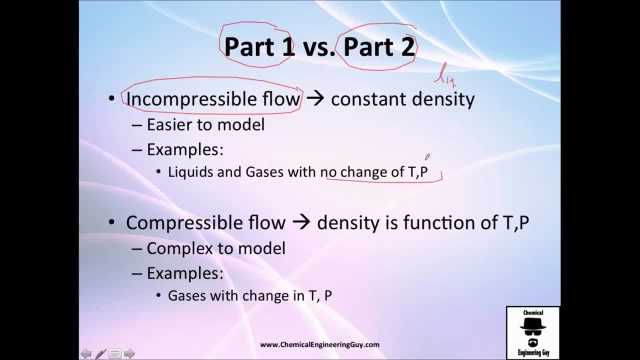 is liquids and many gases with no change on temperature and pressure in its operation, which this is not very common. Normally you change either temperature, pressure or even volume. So you know, with the ideal gas law, if you change any of these you will have something that is not. 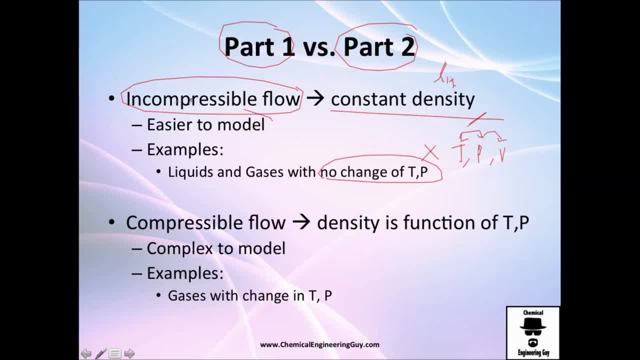 constant in density. The good thing is that this is pretty easy to model, So it's very easy to model it in the mathematical equation. Actually, we're going to use the mechanical energy equation And this is mainly about liquids, So moving liquids. 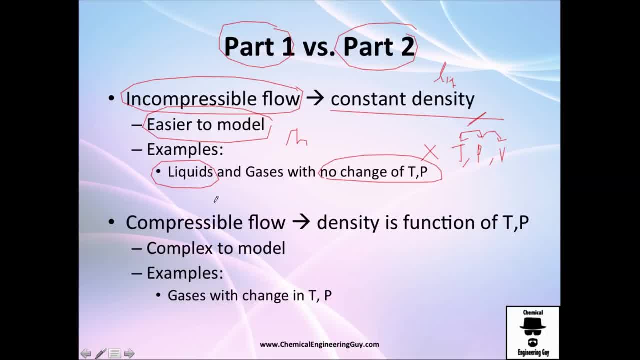 moving and pumping, the height of tanks and friction loss etc. We're going to see that in a little bit. And part number two is essentially just compressible flow, And this is very interesting because we actually have to model density as a function of temperature, pressure and volume. I mean. 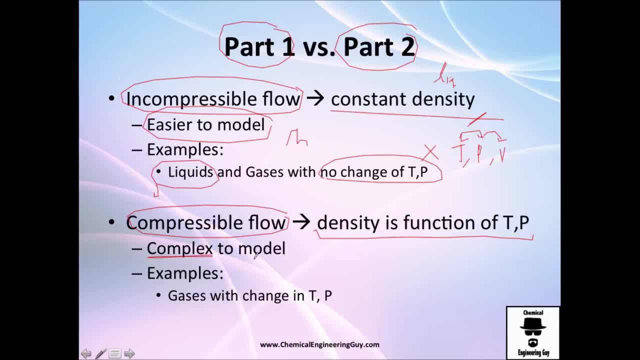 it says complex, but it's actually not that complex. But of course if you compare it with incompressible flow, it is relatively complex. Now examples: essentially moving gases, because moving gases they have friction. When they get friction they increase their temperature. If they increase their temperature, they have 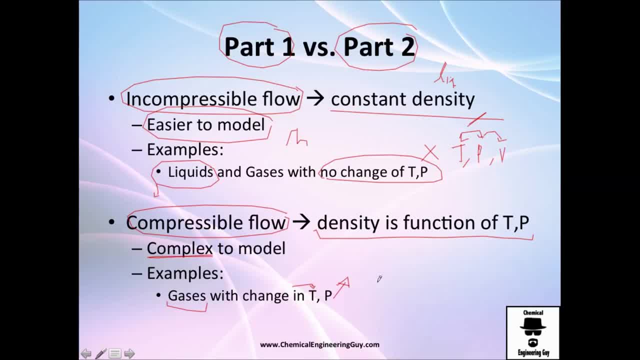 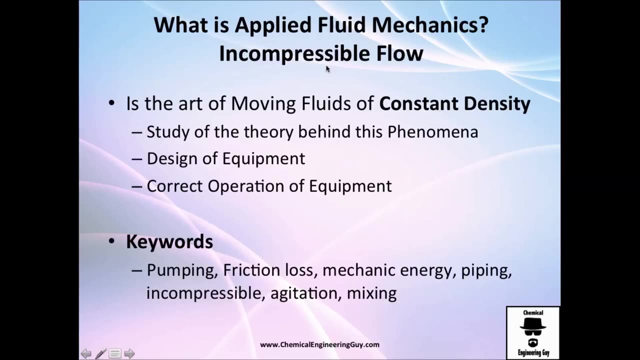 pressure losses Due to friction. the temperature increase makes the gas to expand and therefore you have always a density change with respect to temperature and pressure. So that's why I decided to split the course into part one and part two, Probably if you just want to see the incompressible part or the compressible flow. 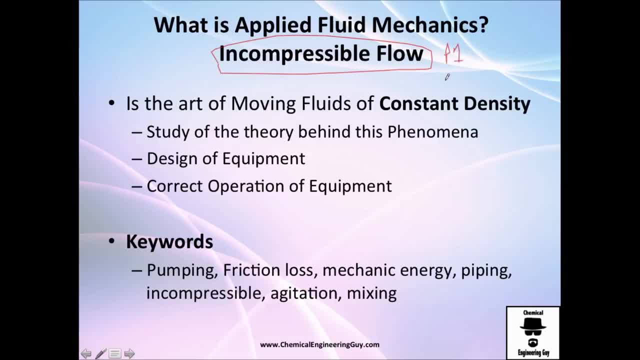 study. you just need to check out part number one. So what's this course essentially about? the incompressible flow is the art- I call it the art- of moving fluids at constant density. So we're going to check out some theory. 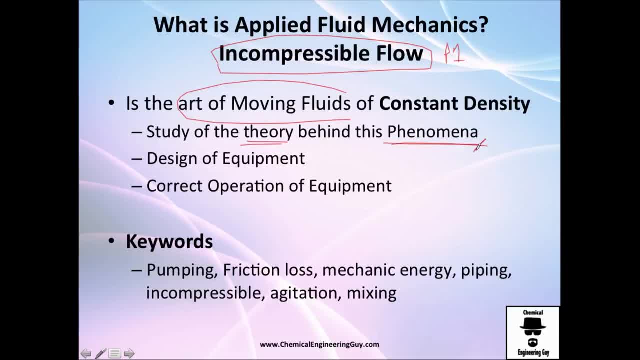 behind these phenomena. You have to check out transport phenomena or momentum transport. You're going to see the application of those concepts in the applied theory or applied examples, real-life problems in engineering and so on. We're going to check out the type of equipments and not only what type of 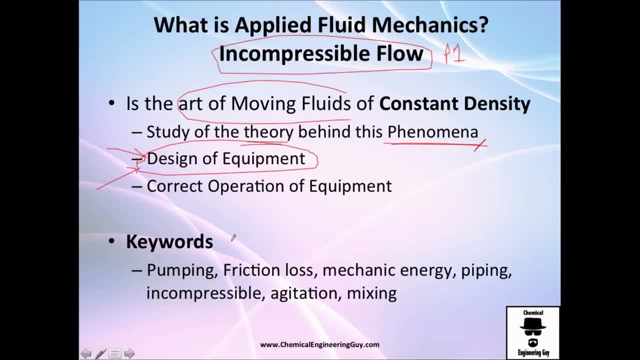 equipments there exist, but also we're going to see or study how to design them and how to operate them correctly. So once you finish this, you will know about pumping, about fluid flow measurement, about friction loss, pressure loss and so on. So the typical keywords you will be hearing or watching and studying. 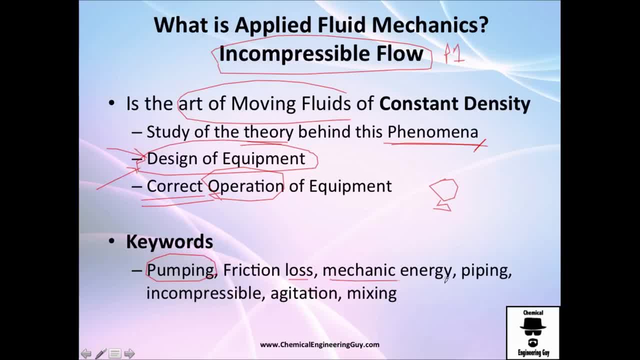 is pumping, friction loss, the mechanical energy equation- Maybe you recall Bernoulli's equation or Torricelli's law. it's okay, we're going to check out this, We're going to study this. We're going to see a little bit on piping and friction. 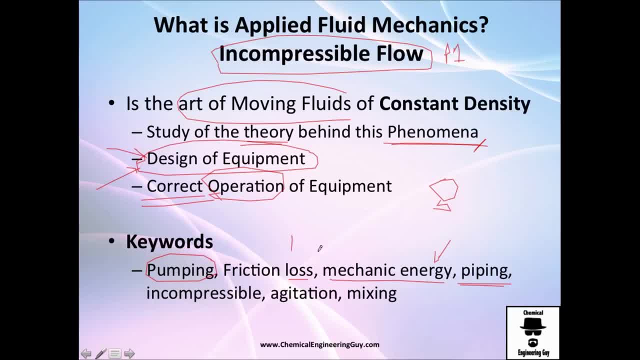 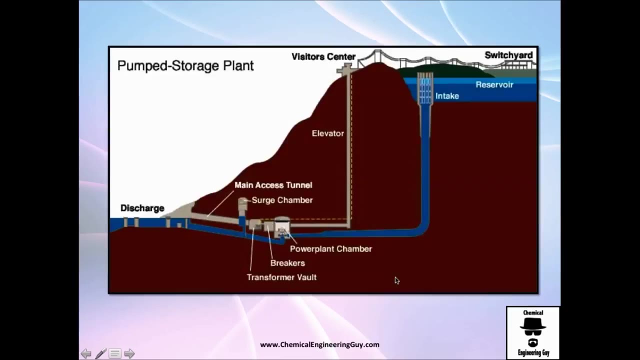 loss type of pipes- cylindrical pipes and non cylindrical pipes- such as this. maybe We're going to see agitation and mixing, which is a very important concept, not only only in compressible flow, but also in reactor engineering. you always need to have a perfect or very good agitation and mixing. so this essentially what's. 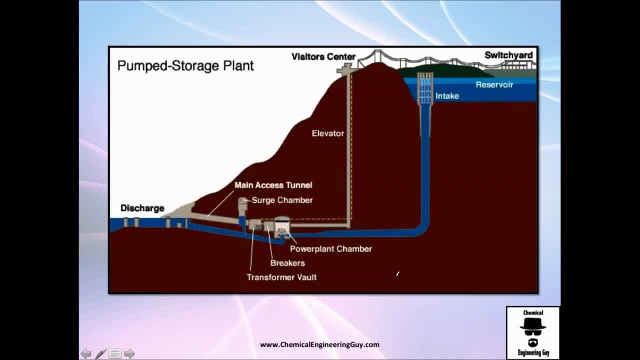 this about. so let me show you a very typical problem that we will be starting is, for example, this operation: we have, let's say we have here a plant that needs to have a reservoir here and it has an intake and we have a discharge, so we use water, let's say, to cool some processes right here and we need to move. 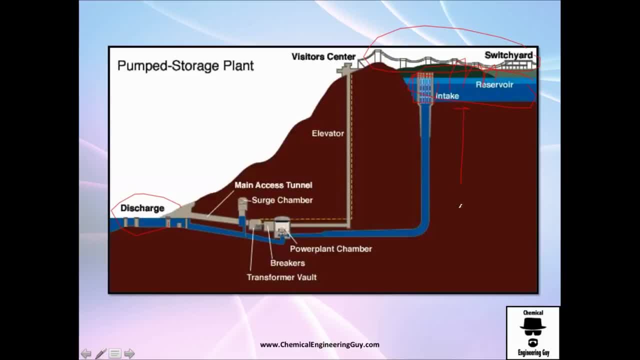 these liquids to the discharge that. you can see there's a height here, so probably you know that the help of gravity, we have no problems. but we also have a power plant here. maybe we need pump because we need. let's say, we have a very high pressure loss so we need to compensate that in order to have in the 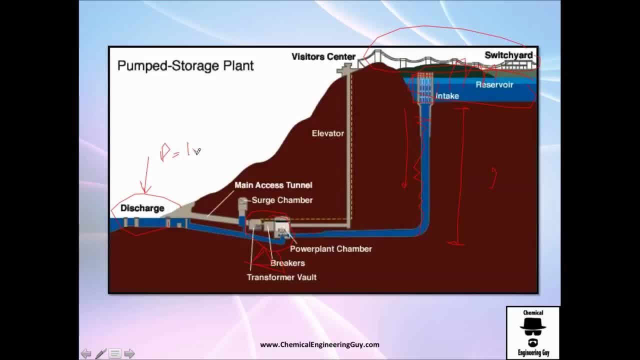 discharge which will have a atmospheric pressure, not only that velocity. we're going to see that many here the velocity. they have different diameters. you can see later that different diameters means different speeds because this is a continuous flow and we're going to see, for example, how much pump energy we need, how much friction loss we're going. 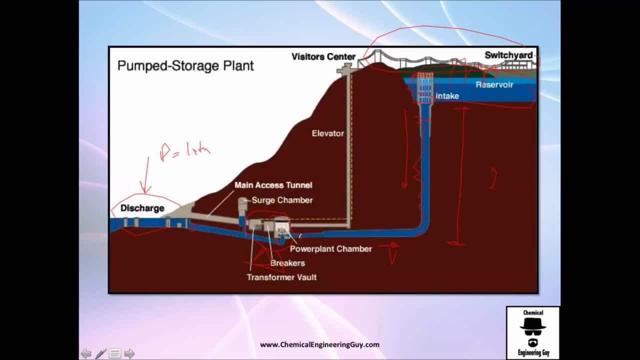 to have. what is the pressure that we should have in the in, let's say here in the suction of the pump and so on? and this one is easy, actually, because you have it here up. what happens if you actually have here the suction and you want to take it to the this here? well, we're going to 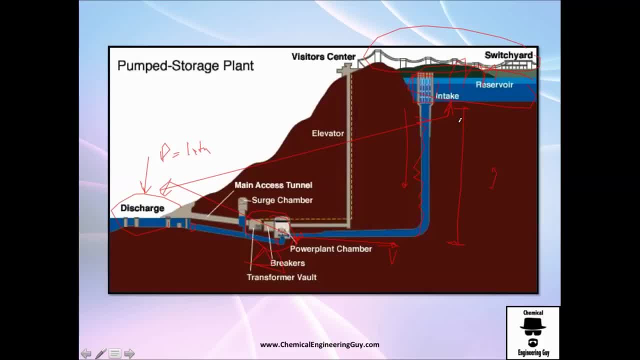 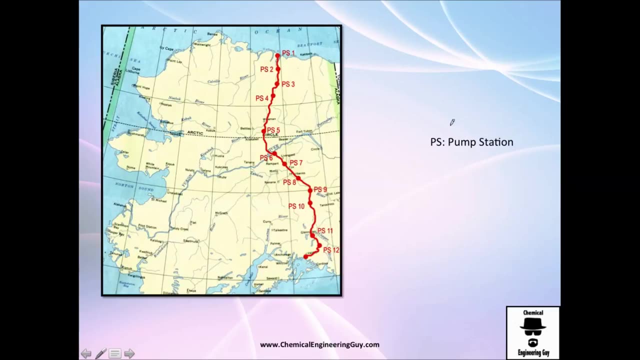 see that as well. this is a very typical example: how to move a liquid from part a to part b and what else i think is essentially everything. let's go to the next one, oops. so why pumping problem? you know this. it's very typical example. we have this. this is alaska, one of the most 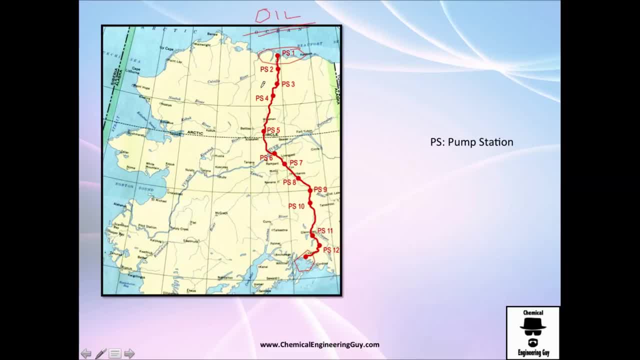 richest oil regions in the world and they have many petroleum here and they start pumping it. you know that by theory, if you want to move a liquid- oops, here you want to move a liquid- you need to add work. it won't move alone and it could probably move along. 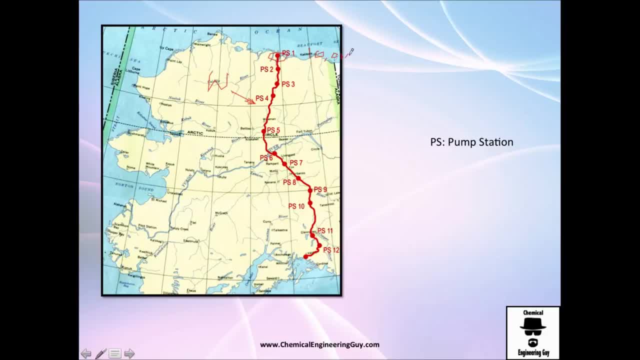 this is what we were thinking and this was, i don't know, maybe 10 000 feet in height, and it was all straight forward to here this point: zero feet, yeah, maybe you could move it, but this is not reality. we actually have no difference on height and we need to pressurize each. 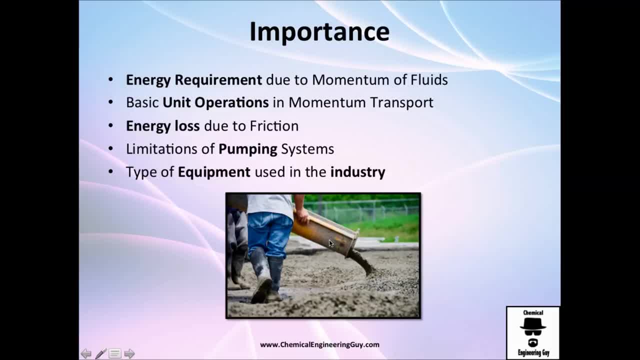 into pump station. for example, pump station 5, 7. actually we have 12 pump stations. so why is it important to move that fluid? We need to know what type of unit operations are needed to do that. Do we need a valve? Do we need a pump? Do we need to measure flow? What's? 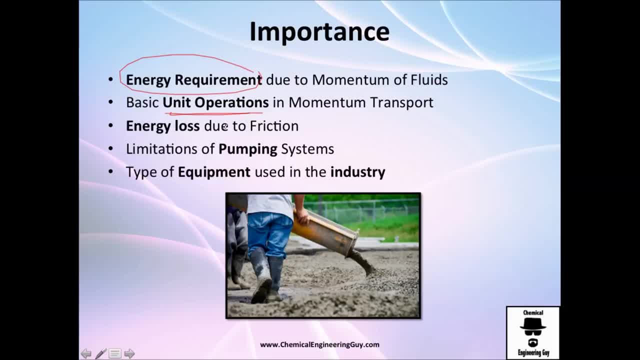 the friction loss of each fitting, each valve, each equipment. We need to know also how much are we losing due to friction, because we know friction is everywhere and we cannot avoid it. but we need to calculate it, to know how much- maybe money- we are going to need or how much pump is required to overcome that. 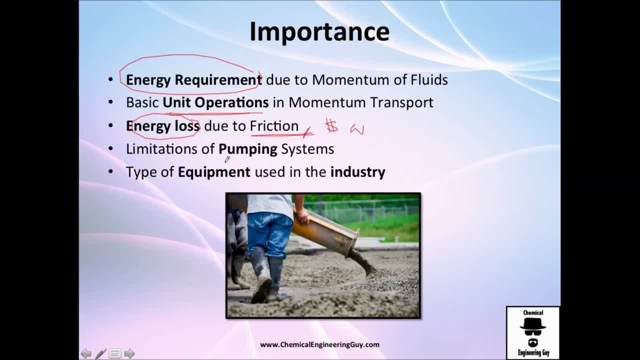 friction loss. And, of course, once you have all this knowledge, you will know the limitations of a pumping system. Maybe if I tell you we have this tank here and we have this little pump and we want to take this fluid to another place of greater height, well, you know that maybe there's a maximum speed flow or 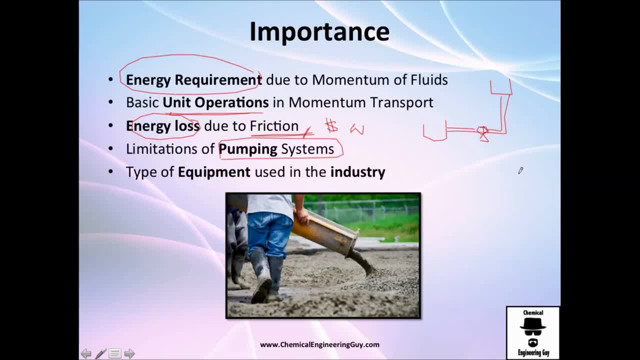 rate that we can operate. So maybe we're working with 10 gallons per minute and you want to check out if 15 gallons per minute is possible or economically speaking possible. So we're going to know the limitations And, once again, the type of. 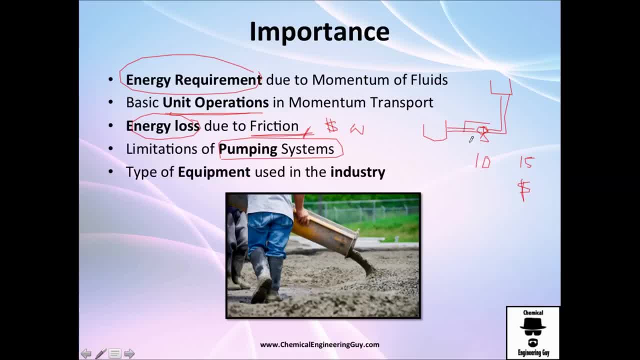 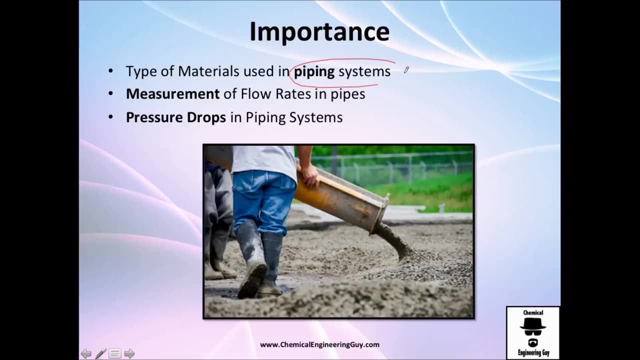 equipment used in the industry, because one thing is what you use in the lab, so, for example, pumping systems in the lab versus the pumping that is actually used in the industry: huge pumps, centrifugal pumps and so on. We're also going to check a little bit on piping. what's a pipe? why we use it. 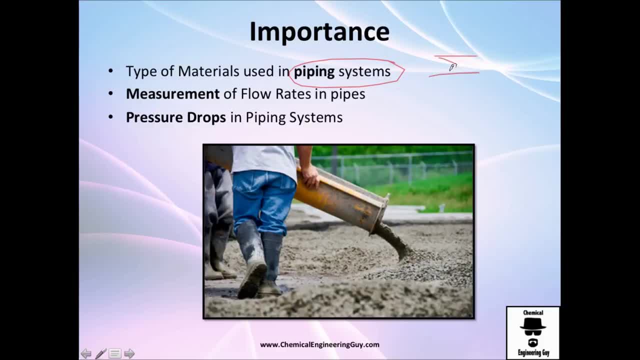 why it's cylindrical: the some profile, velocity profile, this one, there's a viscous profiles and so on. Many type of materials used commonly in the industry: the steel, but there are many other applications such as plastic, PVC and so on. We also check out some important concept on measuring the flow rate. 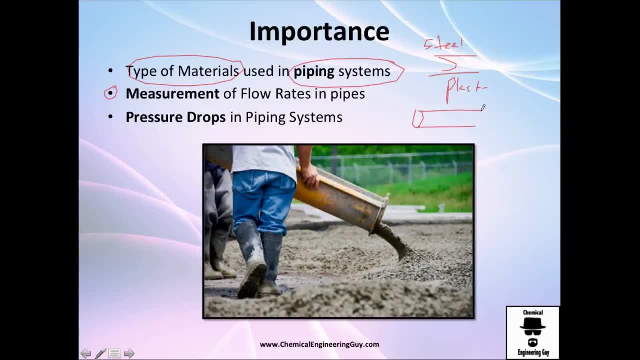 because actually, if you go to a chemical plant, you will see only a tube. You will not see how much substance is moving, and even though you could actually see it, you will need to know the speed of the fluid. So it's kind of difficult to measure it, but we will see. 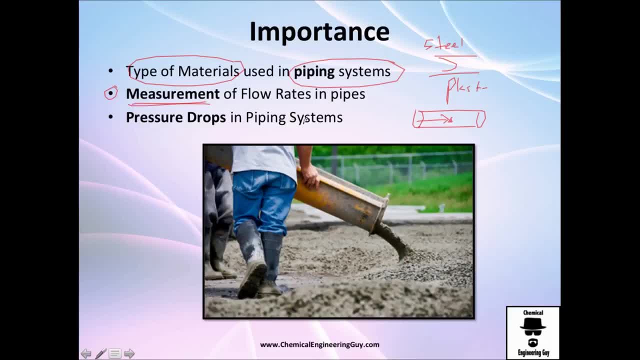 how we can measure that And of course, pressure drops. Pressure drops means that essentially you're going to lose pressure and pressure is essentially force per unit area. So force you also need to work to do that- force moving the fluid. So if we have pressure drop, we 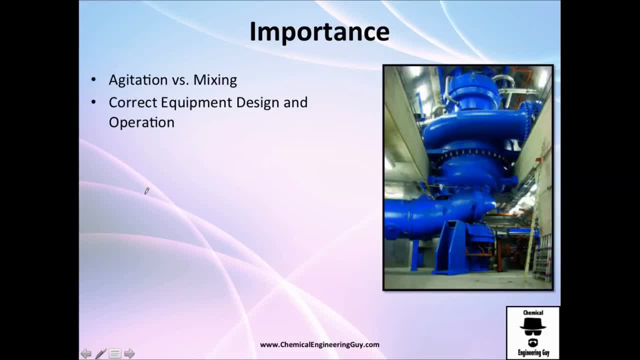 need more energy. Finally, we check out some things on agitation versus mixing and maybe, if you're not an engineer or you don't know this difference, it's actually pretty important to know the difference agitation vs mixing. And finally, the correct equipment design. I mean, when you're doing the numbers, how? 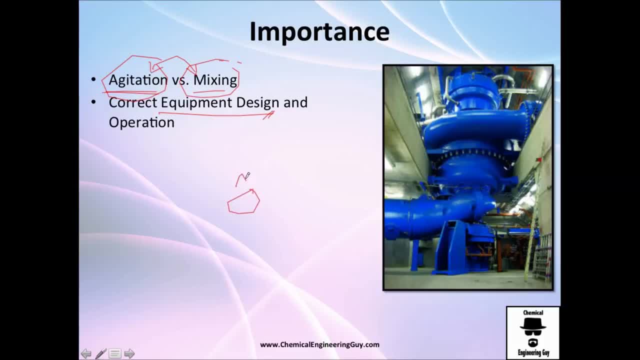 much if you have one task to do. you have fluid in A and you want to move it to fluid or point B, you want to design it and once it's designed- for example, you already have a pump- how can you move, change piping and so on to operate that? is it better to operate the pump at? 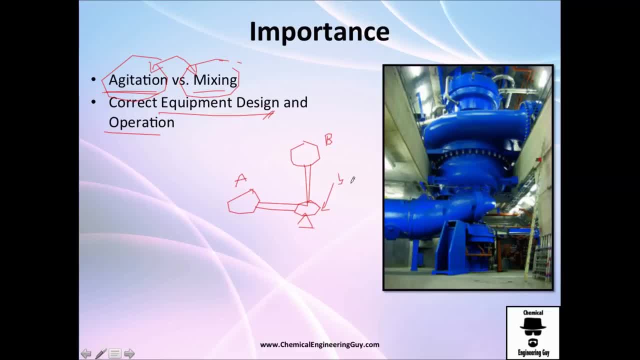 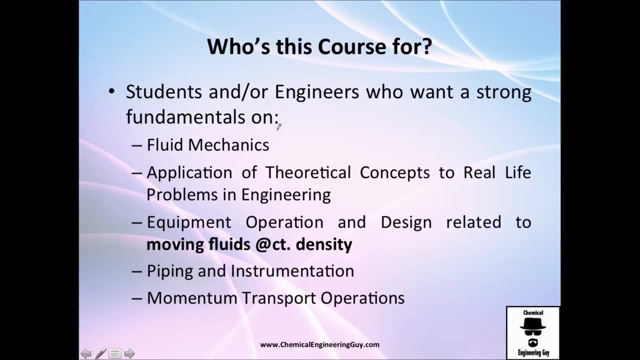 3 500 revolutions per minute, or is it better to check and change the impeller size and what's the better or the best operation point? so hopefully you're getting the idea of what we're going to check and do and study in this course, but if you probably recommend this course for students or even engineers, that one is strong. 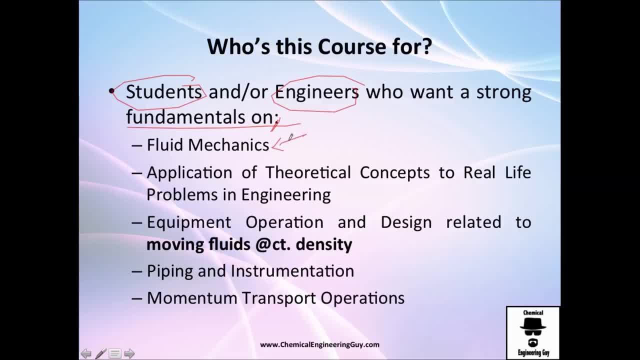 fundamentals on fluid mechanics, essentially fluid mechanics- a theory and as applied theory, i think is very recommended. we're going to check out the theoretical concepts. you're going to check out the theoretical concepts and we're going to check out the, but what this course is about is mainly the application of those theoretical concepts. 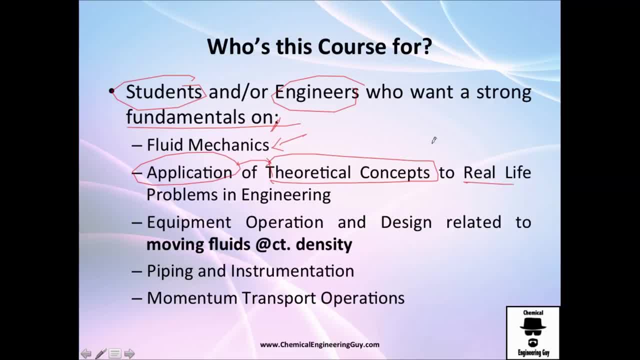 how to solve real life problems. we're not going to see crazy theory. we're going to see the most basic theory in order to solve real life problems. once again, equipment, operation and design related to moving fluids. so one thing is knowing a, let's say, a equipment, and other thing is design it. 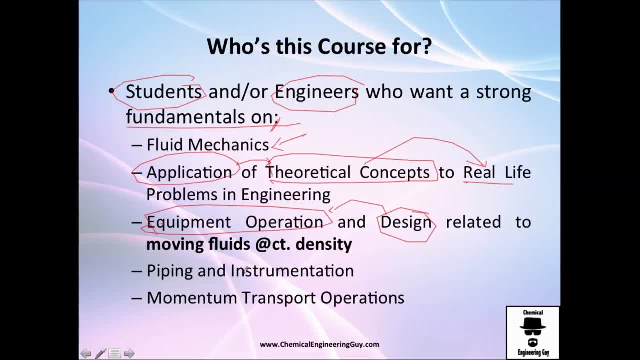 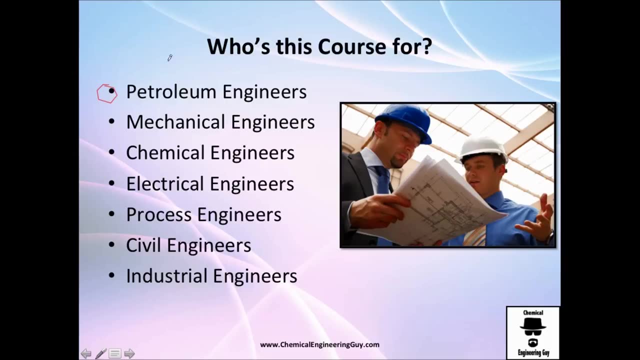 and operate it. we are going to check a little bit on instruments, measurement of fluid rate or rate of fluid flow, and piping. so i will definitely recommend for engineers, especially the ones that need to calculate fluid flow of engineers and need to calculate the pump flow of a very viscous oil or a very 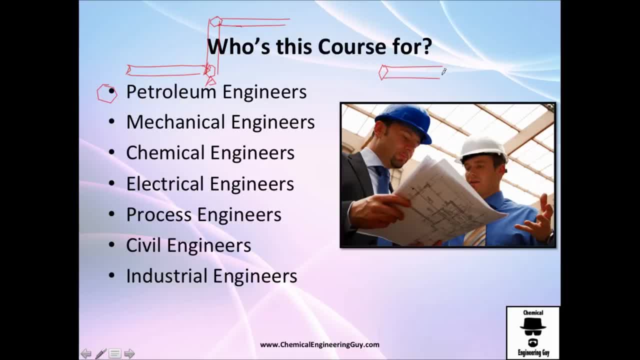 light oil or even gas flow in a petrochemical plant. mechanical engineers: well, because you are going to use pumps and you need to know the change in pressure, the delta p, the pressure needing suction. Chemical engineers: well, of course, if you are in a chemical plant, you 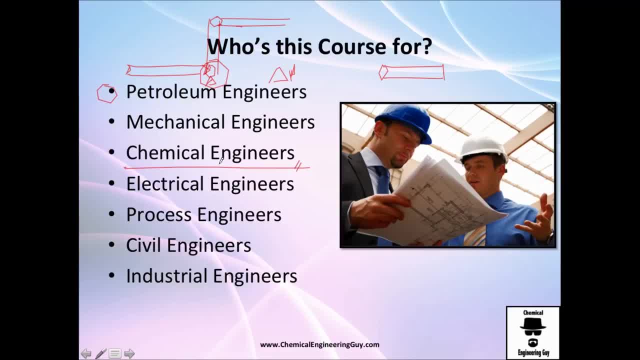 will need it because we need pumps to move fluids and we have many liquids or substances that are in liquid form. so we can use that- Electrical engineers mainly to know why do we need or understand the basics on, why do you have a very high load on the pump or why 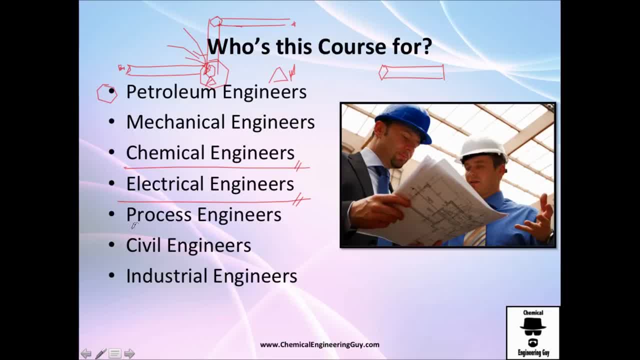 do you have a very low head on the pump Process engineers? well, actually, process engineers. whatever process you do, you are probably going to use pumps or move fluids. Civil engineers in order to have the basics on housing and industries and so on. how to calculate the? 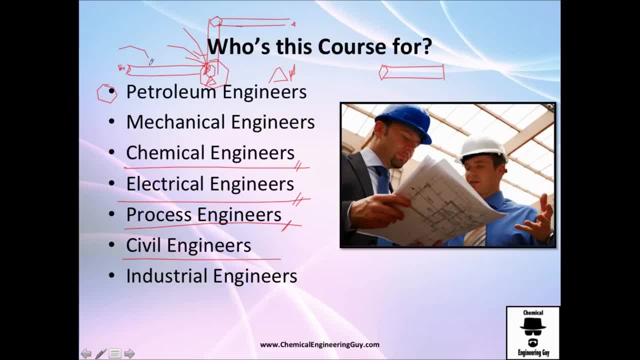 friction loss. How thick should you pump, Should you use the piping systems, How thin, how long, which material? and should you use pumping systems here or in the second floor, and so on, And maybe also even industrial engineers, In order to calculate the amount of energy. is it possible to reduce money, to decrease? 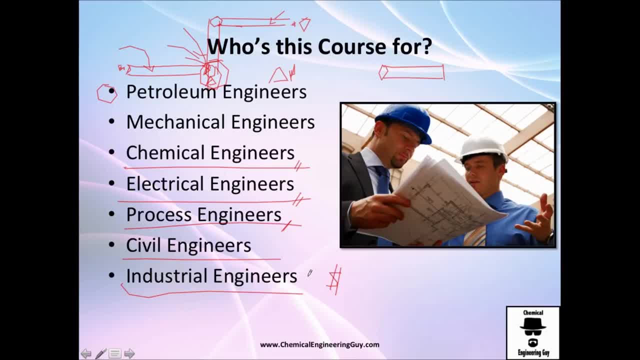 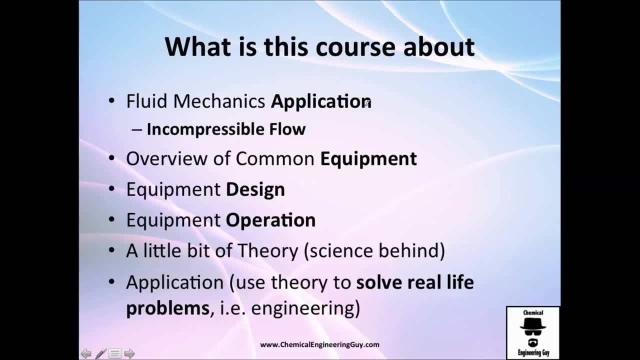 the friction loss or to change the operation of point A or the operation of point B, Nice. So what is this course about? It's about fluid mechanics, but don't see it the way of theory. See it more on the application We're going to see in this part number one: incompressible flow. We're going to check. 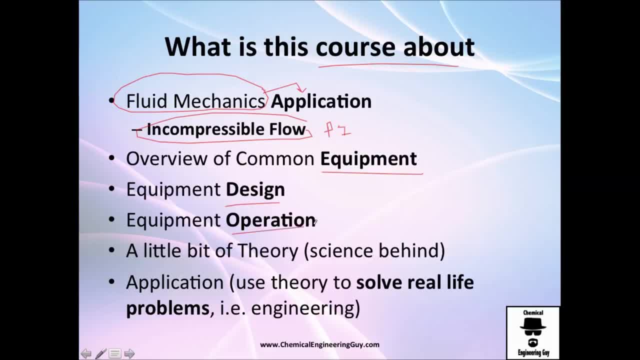 out some equipment, as I told you before, the design, the operation. I mean. this is literally numbers and theory. of course, How do you choose a pipe or the suction pipe? What pressure should you have before a pump suction? Or if you have a series of pumps or parallel arrangement, what's better for you? 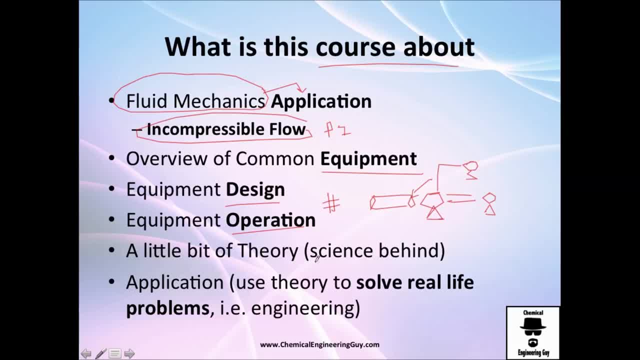 We're going to study that Once again. we're going to see a little bit on science, just the basic. We're not going to study that much on the science behind it. Of course we need to see it because if you don't study that then you will have no idea. 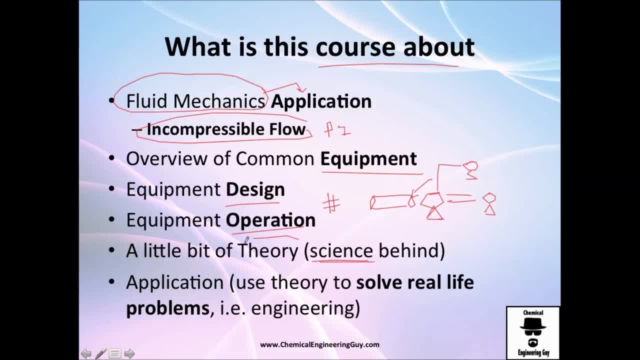 of what we're doing, But I'm going to avoid to go to very theoretical concepts or abstract stuff. And of course the thing here is we're engineers, so we want to solve real life problems. So if you're in engineering, you're probably going to enjoy this course. 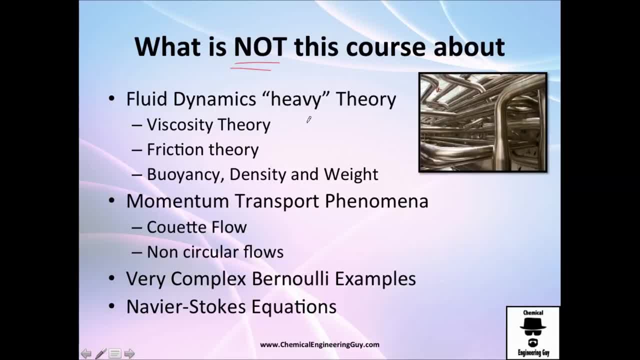 So what's this course not about is essentially very heavy abstract theory of fluid mechanics, For example viscosity theory. why is it more viscous? the shear stress? We have this magical plate moving here to the right, all that stuff that you probably 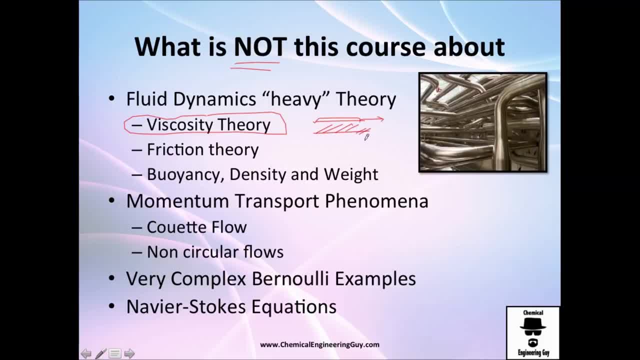 seen in momentum transport or transport phenomena. we're not going to see that. we're not going to see that much into friction theory. we're going just to see the basics, how to calculate it. why does that exist? but we're not going to calculate. for example, calculate the friction of this little drop falling in. 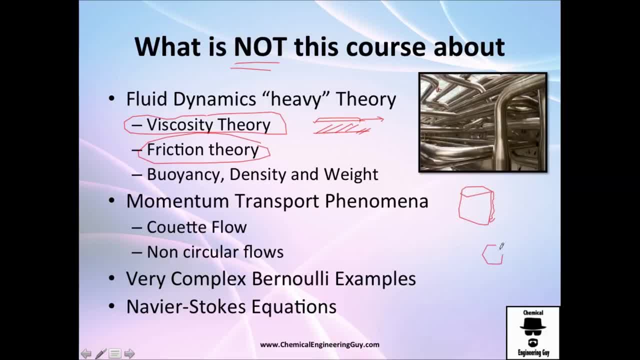 the wall of the cylinder or maybe even the flow, if you have fluid and then crashing the ball, what's the friction? now we're not going to see that, we're not going to study buoyancy density- you should already know it- and the difference between weight and so on. this is I mean. we're going you, I'm going to. 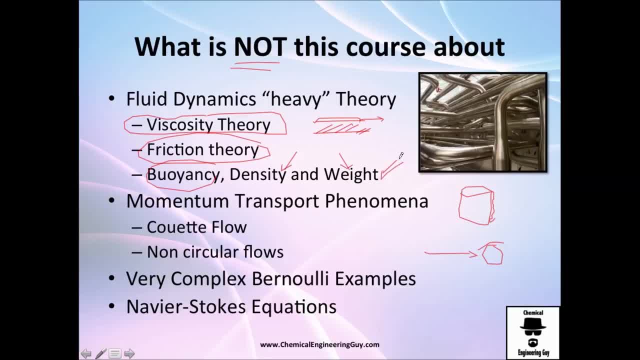 suppose you already have some idea. so you have at least the basic idea, it's okay. now we go to momentum transport phenomena. as I told you before, this is actually co-ed flow. we're not going to see that. oh, you know, it's very good, you know it. if you don't know it, it's okay. 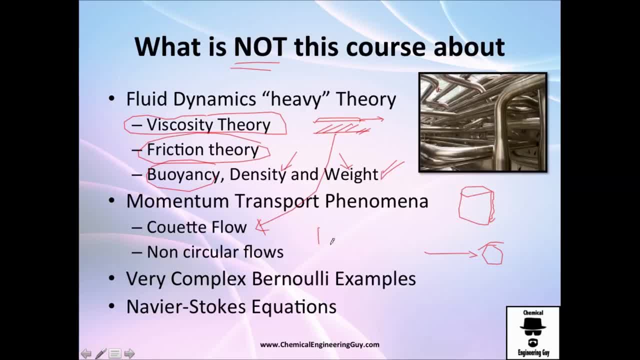 you don't need it. non-circular flows, for example, very crazy ones- I mean we're going to see some, but just the basics. but for example, this flow, calculate the- I don't know- the shear stress in this wall, or maybe we have this pipe and they. 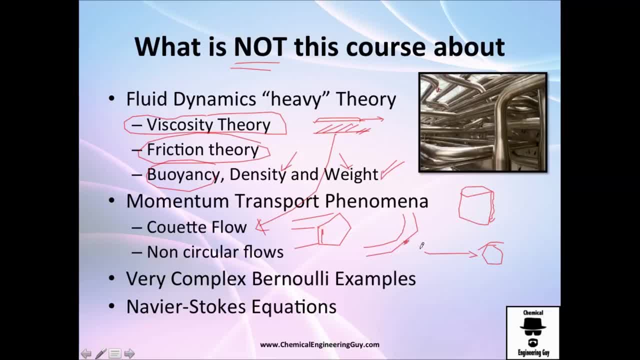 tell you calculate the stress on this point. right here we're not going to see that very complex Bernoulli examples, because I could literally show you many crazy examples on Bernoulli, but actually if that doesn't work, then I'm not going to show you how to calculate the shear stress on Bernoulli, because I could literally show you many crazy examples on Bernoulli, but actually, if that doesn't. 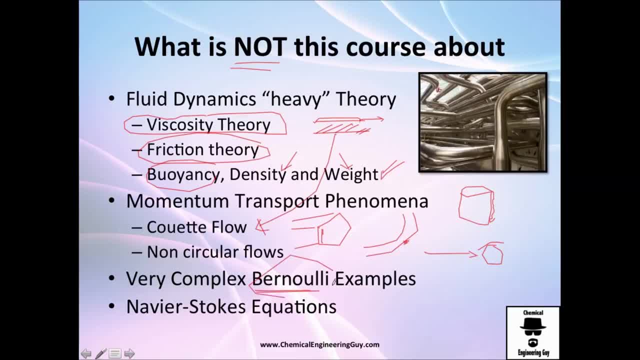 not happens in real life, why would you want to do it? I mean, yes, you can model very crazy stuff, but if you don't apply it in the real life, no, I don't see the points that much, at least not in engineering and Navier-Stokes equations. 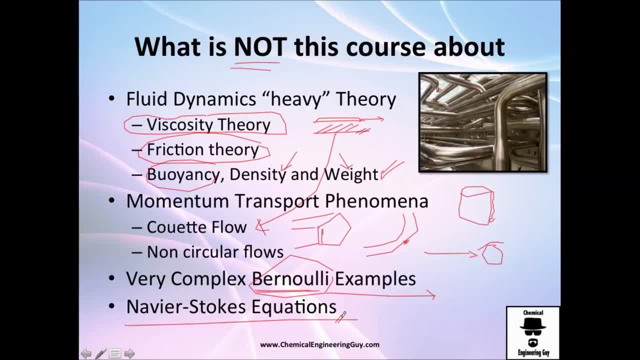 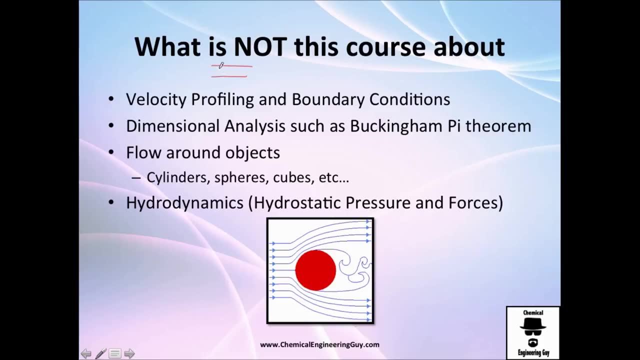 all those crazy equations that talk about fluids and laminar flow. we're going to check out laminar flow, but essentially what we operate in the industry is turbulent flow because we want high speeds and, once again, velocity profiling. we're not going to check out the profile. I. 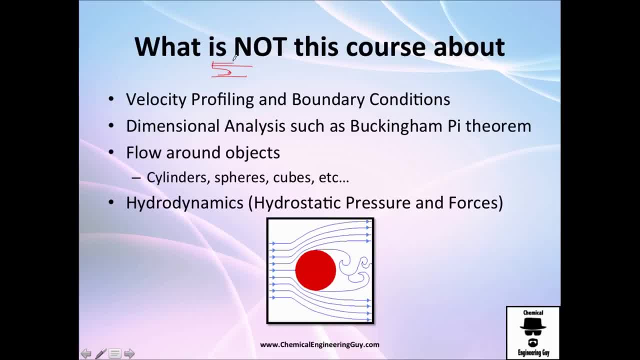 mean like, for example, how is, how long is this length? or is it plug flow and so on. we're going to see a little bit in that, but we're not going to model that. we're going to see the theory and some, for example, examples, but we're not going to 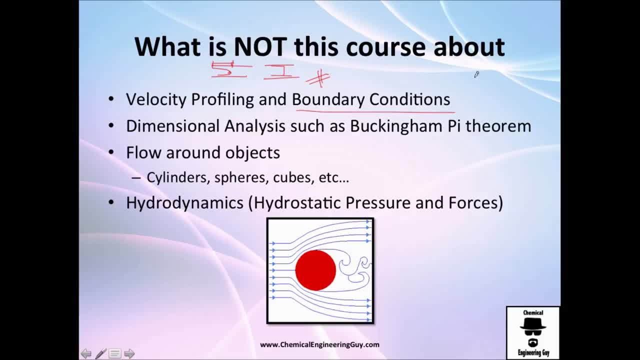 do numbers in that and the typical boundary conditions, which is very common in transport phenomena. they tell you they, you have the radius and you have these shear stress and the viscosity is actually zero, velocity is equal to 0 and so on. we're not going to see that Also. 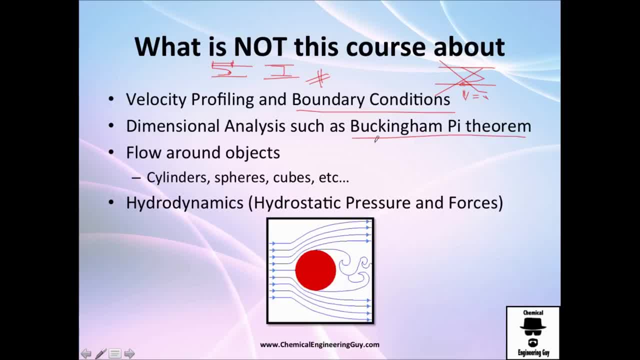 dimensional analysis, such as the Buckingham P theorem or Pai theorem. no, actually, actually we just use this for Reynolds number and relative roughness, and you don't actually need to know where does these numbers come from. you just need to know how to calculate them. Flow around objects. 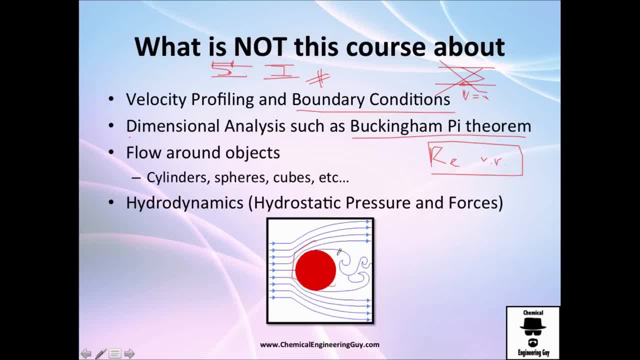 cylinder, sphere cubes and so on, for example, this stuff. well, we're going to see an example, but we're not going to use numbers, and we don't. i'm not going to ask you what's temperature right here or what's the number right here, and i'm going to suppose that you already know a little bit. 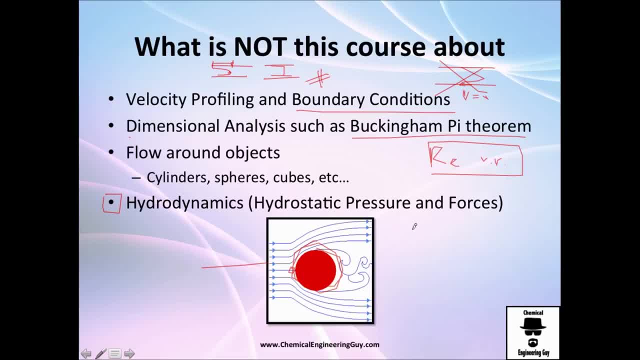 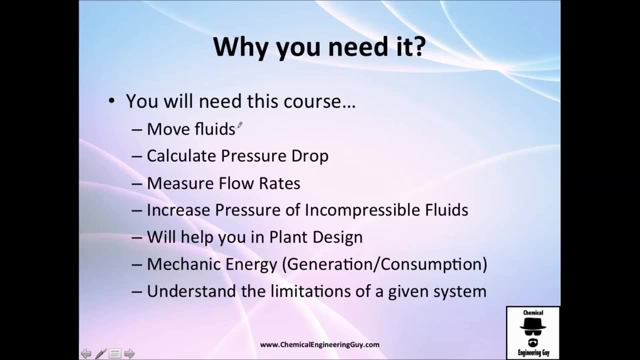 on hydrodynamics, which is hydrostatic pressure and forces acting on this, which is very common in high school, middle school and even physics courses in bachelor degrees. so why you need it? essentially to move fluids if you task- i know it sounds kind of stupid moving fluids, but actually there are many people working on this. if you need, for example, to move 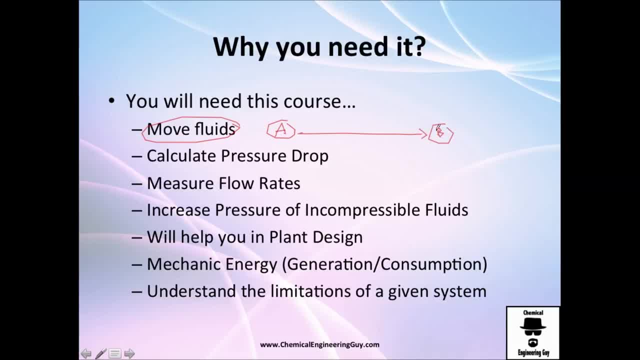 a fluid from point a to point b. how do you do it? what's the best way? should you use a pump here or a pump right here? should you elevate this point? can you depress this point? if we use this material, we have this friction loss cost, but it's very cheap. 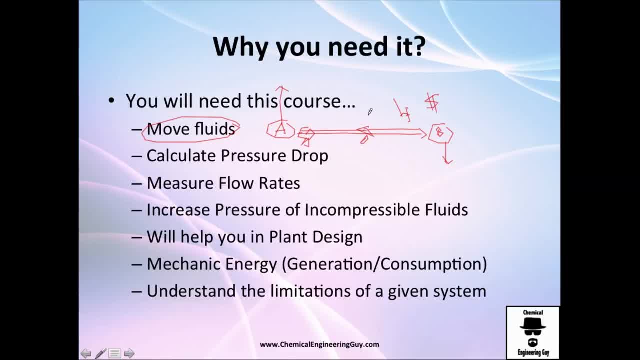 so it's good to for the investment, or so on. we will also need to calculate the pressure drops in order to calculate the size of the pump. we also need to measure flow rates, because we cannot be producing without knowing how much stuff is going in and going out. shall we increase the pressure? 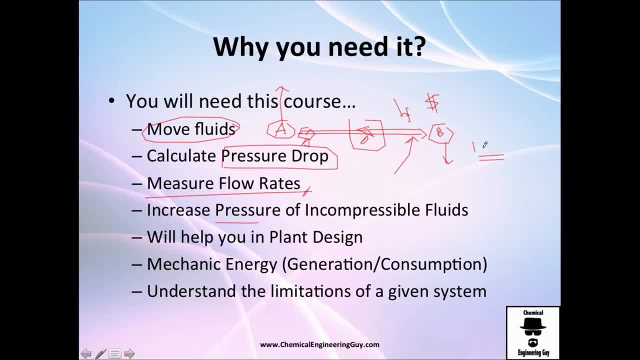 for example, many times you need to operate, you have a pressure at one atmosphere and many times you want to send this fluid to a distillation column which operates at three atmospheres. well, the engineer, the distillation engineer, tells you: i need this fluid at three atmospheres. well, 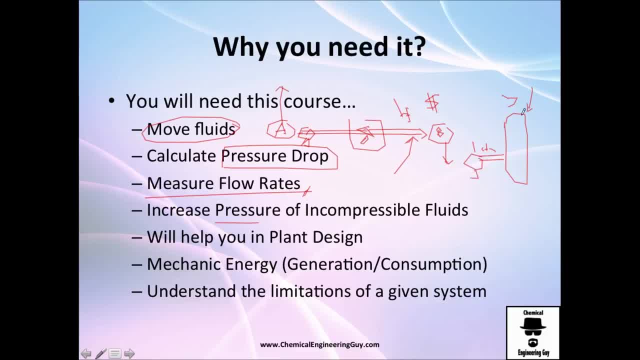 even though you don't know why you need to do it. one atmosphere to three atmospheres will definitely help you in plant design. we're going to use as well the mechanical energy equations, so how much is needed and consumed, and so on. and, most importantly, once, many times you go to a chemical plant or 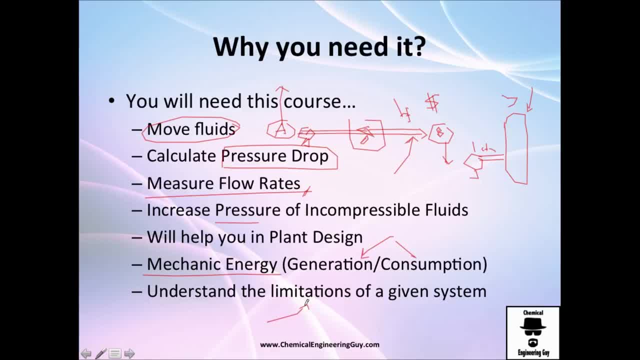 anything that has a pump or pumping system and it's already done, so you cannot move. the piping system is done. the point a and point b is already set. you cannot move it. the pump is there. uh, you're gonna change anything but valves and operation of the pump leg, the size of the impeller. 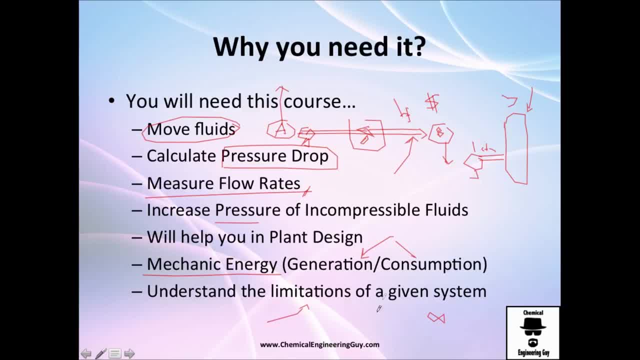 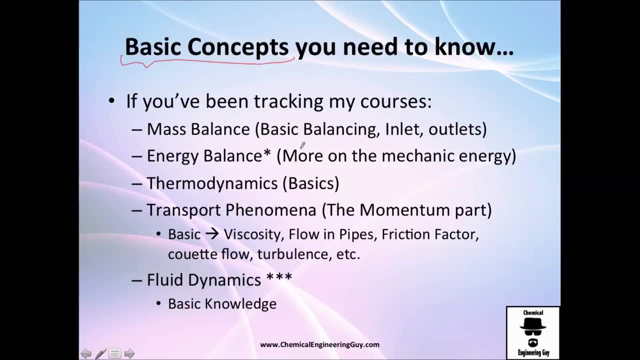 and so on. so how, given that, how can you actually play with that in order to get the best economic or technical operations conditions? so what i'm going to ask you to know is essentially: you've been tracking my courses. i have a course in mass balance. essentially, we're going to use just the basic balancing in that outlet. we will have no reactions. 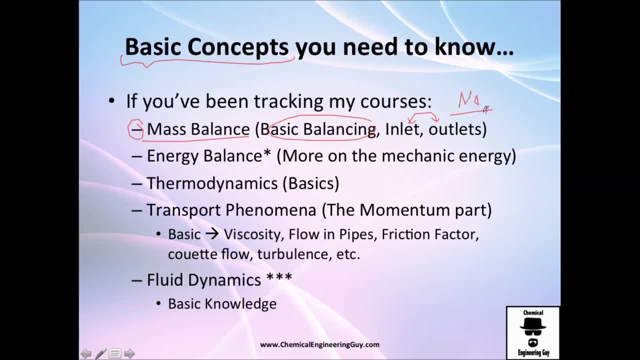 we're going to have, of course, only moving fluids. energy balance, just the basics, especially the mechanical part. i'm going to do a course on energy balance, but this is more on the heat requirements. actually, this is the good course because we use the mechanical part, because, you know, energy is. 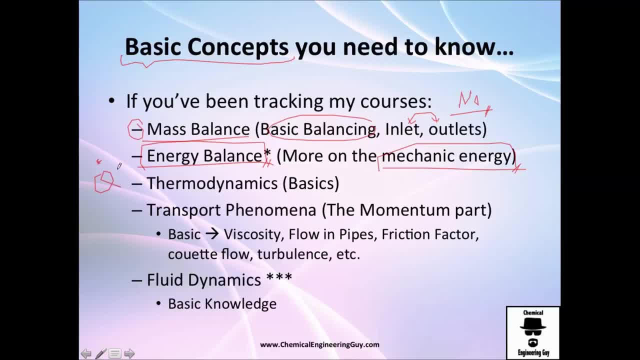 either heat or mechanical energy and energy balance. we check out heat and in this course we check out work and we use the mechanical part. so we'll see how we can modify the electrical part. so the basic things that we need to do here is just the basics on thermodynamics, essentially. 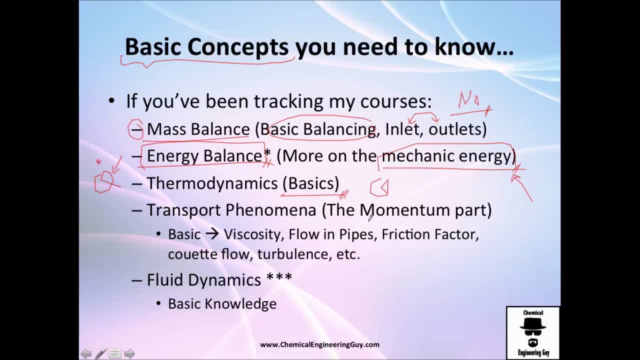 why do we need to heat material? why do how to model ideal gas loss, how to model real gases and so on. a little bit on transport phenomena, especially the momentum part. just the basics. what's viscosity? uh, flowing pipes, friction factor covet low turbulence, even though between kinematic viscosity dynamic. 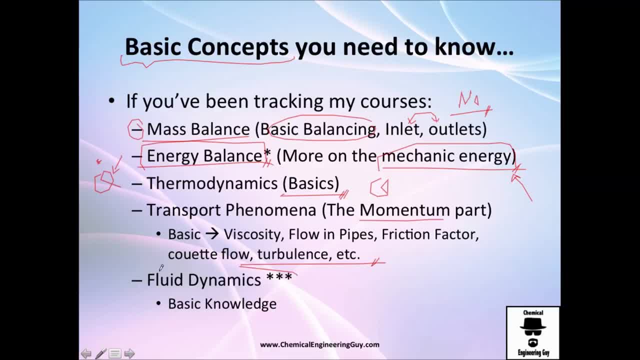 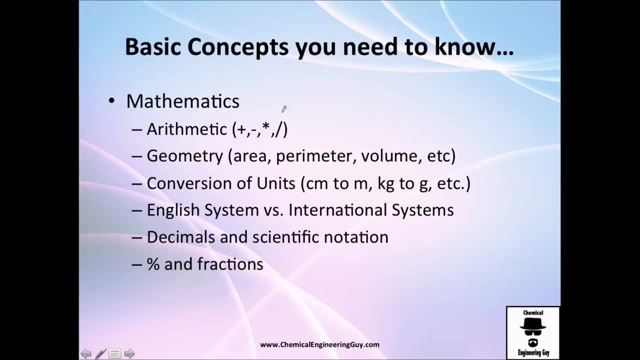 and so on And fluid dynamics, just basic knowledge actually, just to know that pressure, how do you measure pressure in a pipe, and so on. It's okay, we're going to see all through, so don't worry For mathematics. actually, you just need to know the basic arithmetics, please. 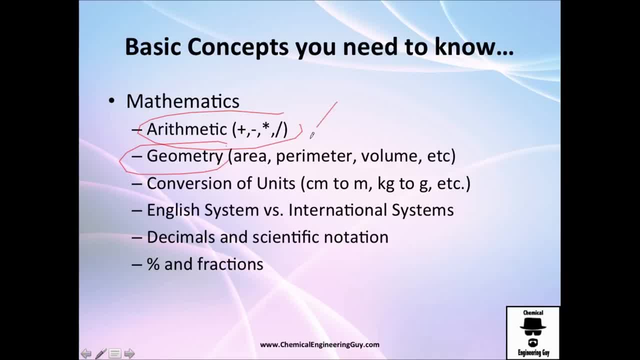 be sure to know the geometry. because when I tell the students you just need to know the area and perimeter and volume of, I don't know, a circle, a sphere, a cylinder and so on, and they tell me, yeah, it's pretty easy. and then you get into the numbers. you ask them: what's the perimeter of the? 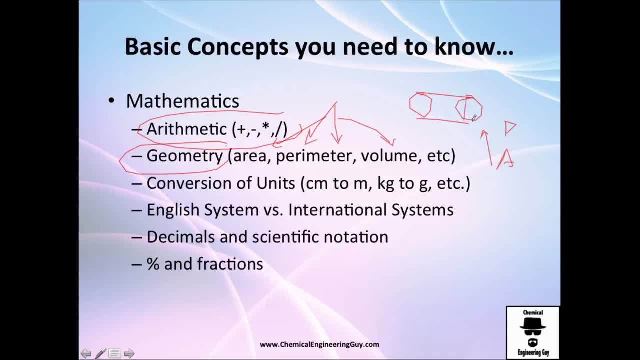 cylinder and you ask them what's the area of this pipe and they don't know how to do it. so please be sure, even though we're going to check this out, just be sure to know it. Conversion of units is very critical in this course, not only from SI system. 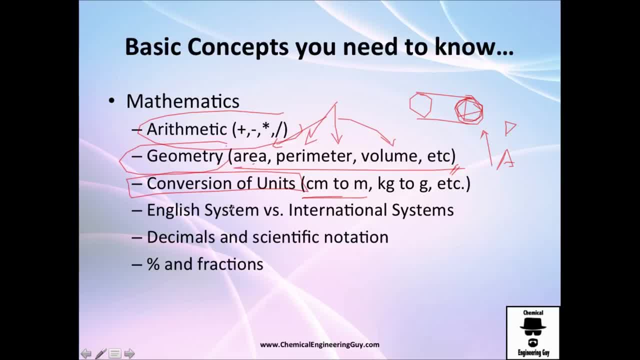 but English system to international system, for example, Fahrenheit to Celsius, pound force to Pascals or Newtons and so on. Well, of course, decimals and scientific notation and how to use fractions, But actually, if you ask me, what's more important here is the geometry. 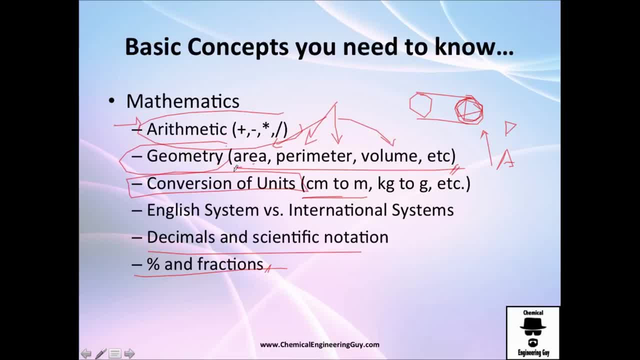 have a good basis in math- which I probably know you have because you're studying engineering or something related to this- and please be sure to use the English system and know a little bit on the English system. If you are an English system native user, well then you will have a little bit. 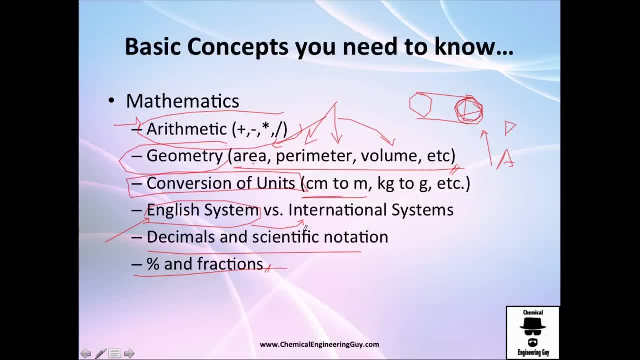 problem when you change to international system. and my recommendation essentially is for the SI system users, which is essentially ninety percent of the world is just to know the conversions, just check out what the conversion and go back to international system. use the most logical system here which is very easy to use. 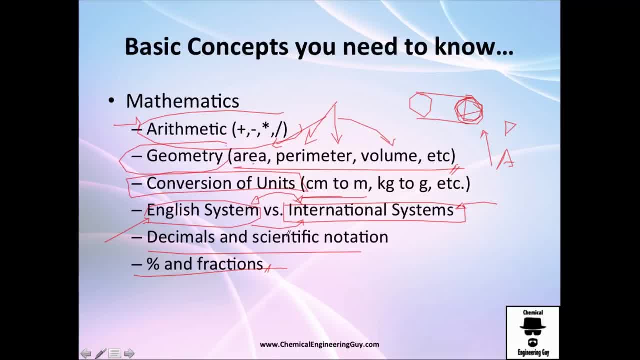 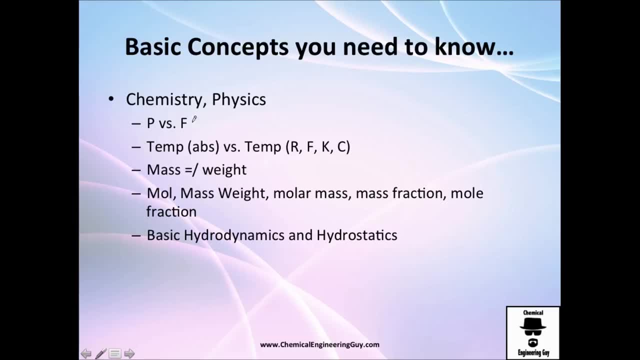 and forget all the complex English system conversions. What you need to know in chemistry and physics is just, for example, pressure versus force. please know the difference. how to change absolute to normal temperature, for example, Fahrenheit to ranking, Celsius to Kelvin, Celsius to Fahrenheit, Fahrenheit to Celsius. 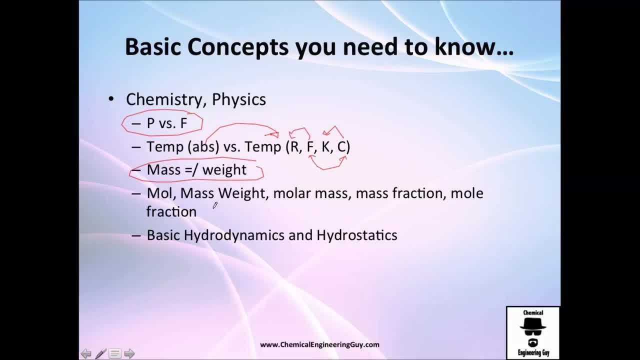 and so on. Please know what's the difference between mass and weight. what's a mole? mass weight, molar mass, mole fraction- all this stuff that, for chemical engineers, is actually very common. maybe you're a, let's say, electrical engineer. you have no idea. well, please check it out. this is 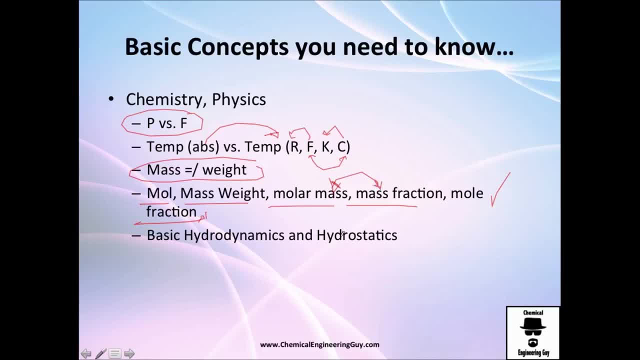 literally basic chemistry. check out your high school notes or even, I'm pretty sure, in YouTube. there are many videos on how to calculate moles from a molar mass And basic hydrodynamics and hydrostatics. just know that the column exerted by a fluid, this is the height. 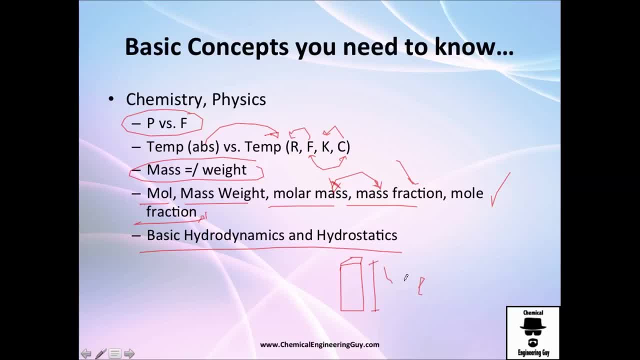 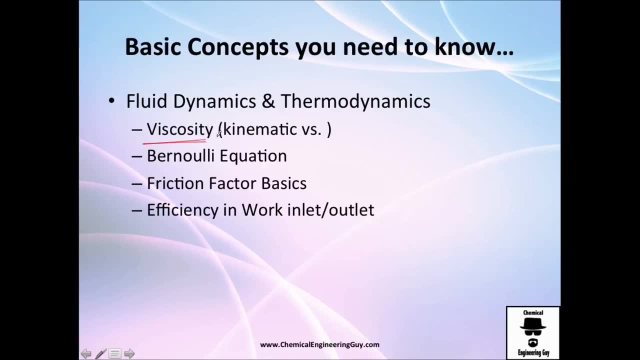 you know there is a density and gravity. well know how to calculate the pressure exerted by that fluid. Once again, viscosity. but we're going to check it, don't worries. the Bernoulli equation: I'm pretty sure you have heard or even used it, so if you have used it before, 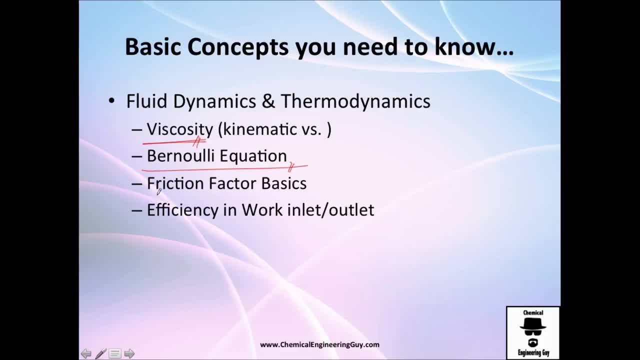 you're going to have a advantage: Friction factor, basics. if you don't have what's, if you have no idea what's this about, No worries, we're going to check this out very deeply and How to calculate the efficiency in work. for example, the efficiency for a pump is different for a. 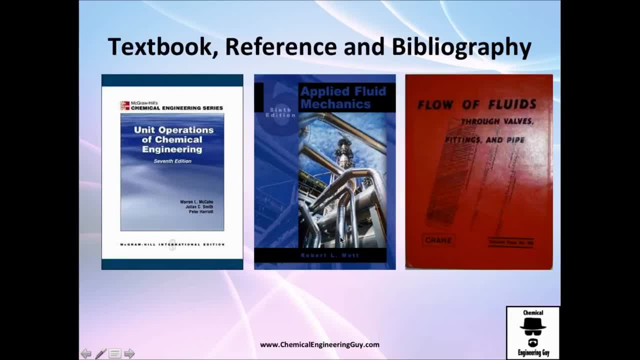 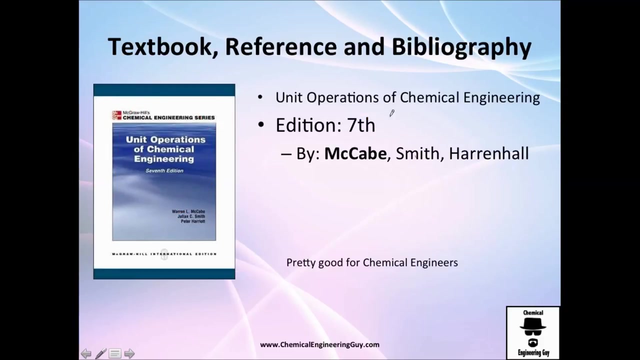 efficiency in a turbine system. Good, now let's check out books. I will be using essentially these two books for theory and exercises and examples, and this is mainly for fittings, pipes and valves. Friction- essentially for the friction part. Let's check out. I'm pretty sure this is the seventh edition actually. 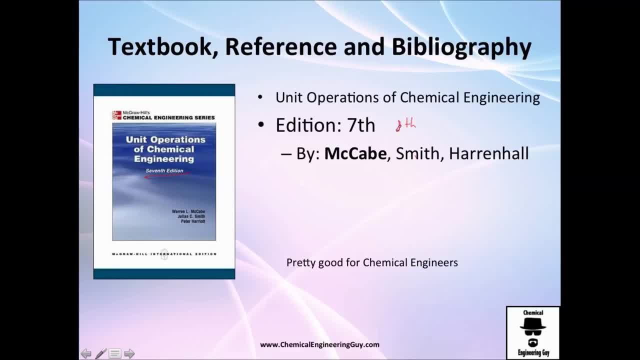 Yeah, seventh edition, but I think there's already the eighth edition. You can use whatever you have or want. It's unit operation of chemical engineering, essentially Unit operations, you know it's. it's like pumps, compression, piping, flow measurement and so on. It's done. It's written by McCabe, Smith and Harald. This is a pretty good. 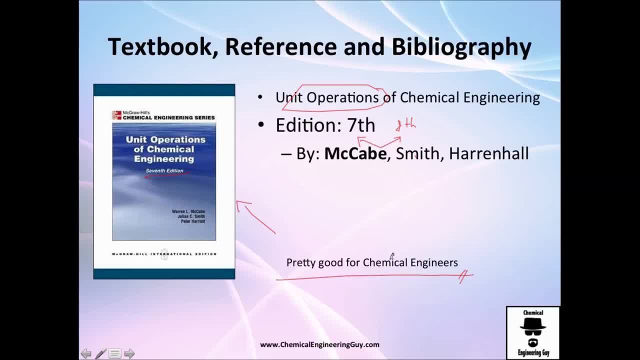 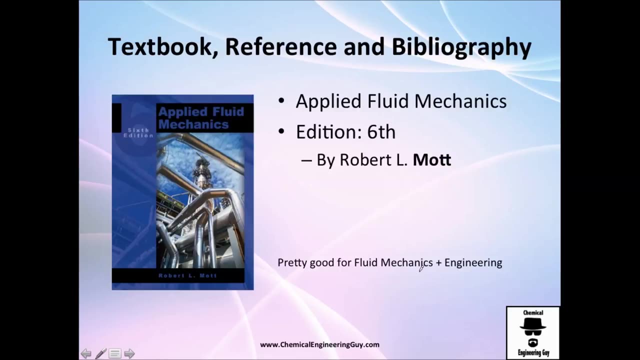 Book for chemical engineers and even for- I will say, essentially for- engineers. We're going to check out many Chapters on this book. I'm going to show you which chapters we're going to see: study problems and so on. Now the- as the name implies, I actually love this book because this is essentially 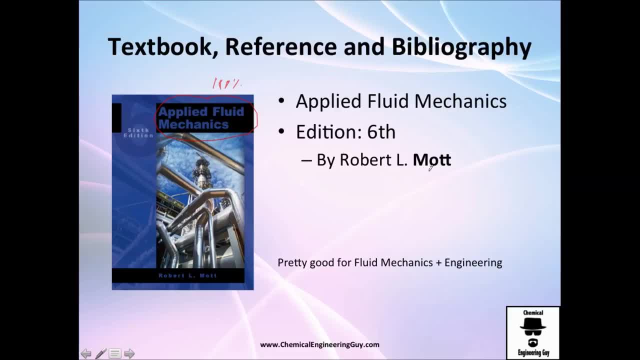 100%. our course is applied fluid dynamics by Robert L Mott, sixth edition. It's pretty good essentially for any fluid mechanics because you have many theory behind that And we have a lot of application of that theory. We're going to check out that. I 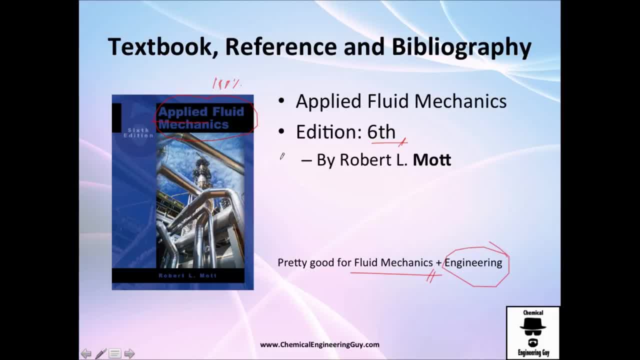 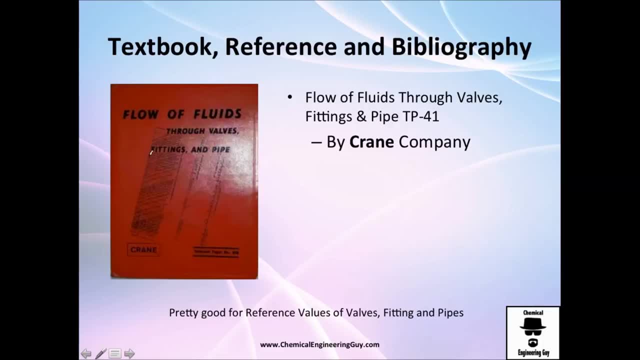 Would definitely recommend for any engineering field related to fluid mechanics- And once again this is the flow of fluid through balls, fittings and pipe- is essentially just for the friction data. There's no, not that much theory, but actually it's very good for a reference book. 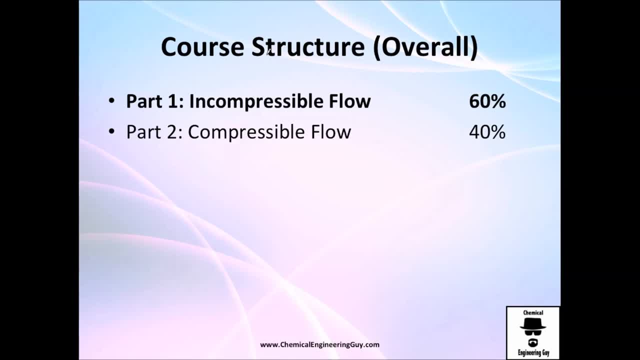 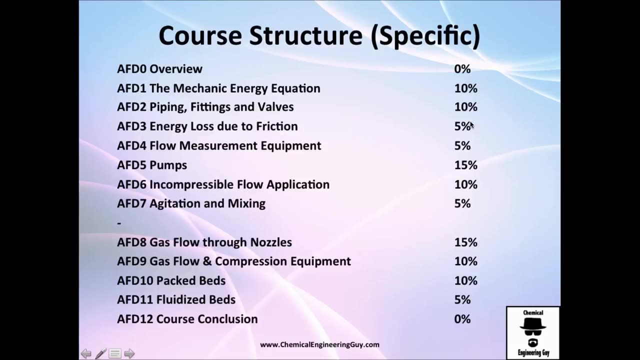 So let's check course structure. Remember this is applied fluid dynamics course and we have it in two parts: parts number one, Which is incompressible flow, and part number two is compressible flow, 60 and 40 percent each. So, for instance, this is part number one and this is part number two. 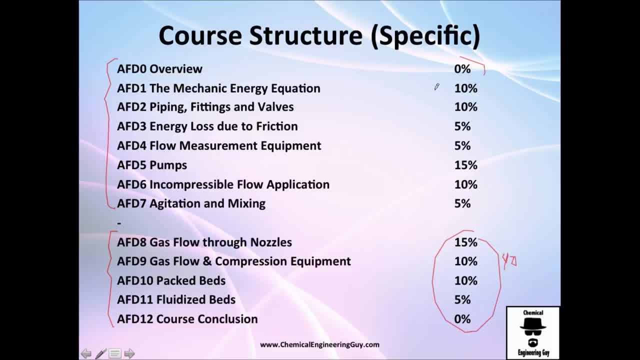 If you check out this is about 40 percent and if you check out this part right here is 60 percent. Okay, this part number two. you are interested in gas flows, Gas flow the room, us Els, tubes, typing's and compression, And also operation such as pecbed and fluidized beds. Please check out part number two. 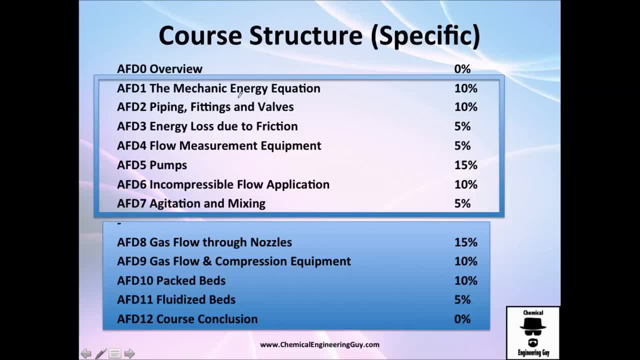 Part number one will be essentially just in the repluck, the Mechanic Erie equations. we're going to see this a Little bit more in the next slide, So let me show you guys. these piping fittings on balls is just theory. energy loss due to friction: 5%. flow measurement, 5% pumps, 15%. actually, this is. 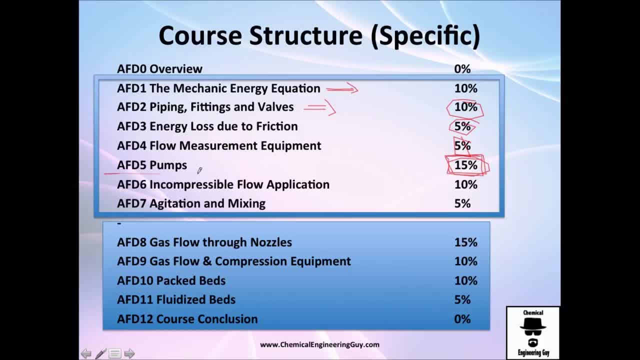 very huge amount of material, and this is one of the core blocks. then we go to incompressible flow application. once you know all these, you know the mechanical energy equation, how to calculate friction losses, the type of pipes, fittings and bulbs that there exist and flow measurement equipment, and you know 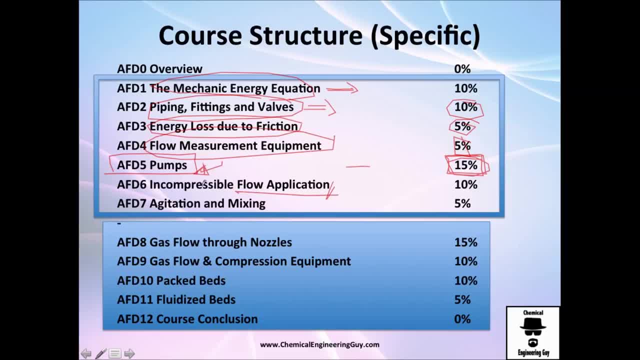 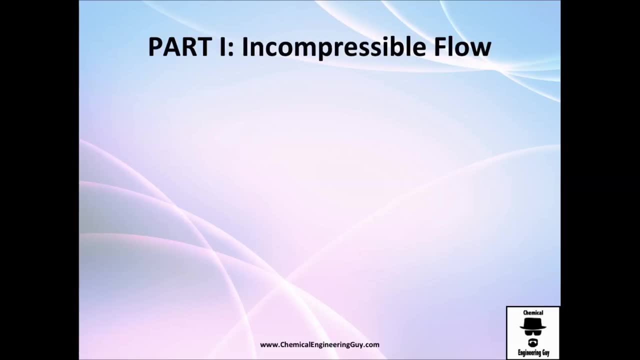 finally, how to choose a pump. we're going to check out incompressible flow application- so many real-life problems- and how to solve them here and at the end we check out a little bit on agitation and mixing. so let's see a little bit more content on part number one, incompressible flow. but before 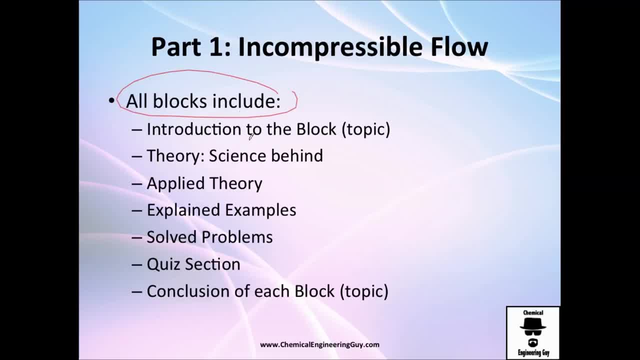 actually checking out each block. I just want to tell you that you will always find a introduction to the block, so you don't waste your time, you just check out and if you think it's very useful to you check it out, you will check or see what's the best part. 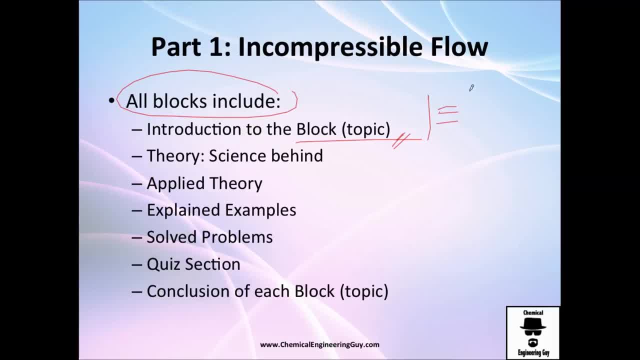 for you and go on. so you don't need to actually study all the block. you just go here, see or check out what's useful for you and go direct to there. now the theory behind. we're going to see the theory and then we're going to apply the 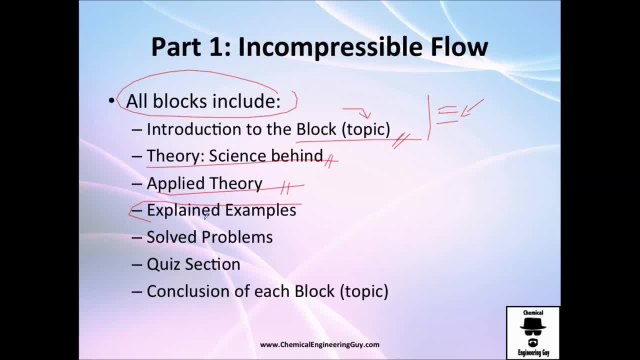 theory for real-life problems. we're going to have also explained problems. I mean with numbers and using the equations and so on. solve problems are included in the webpage, so check it out. we're going to have also a quiz section which is essentially just theory: pop quiz, for example, a 50 questions on 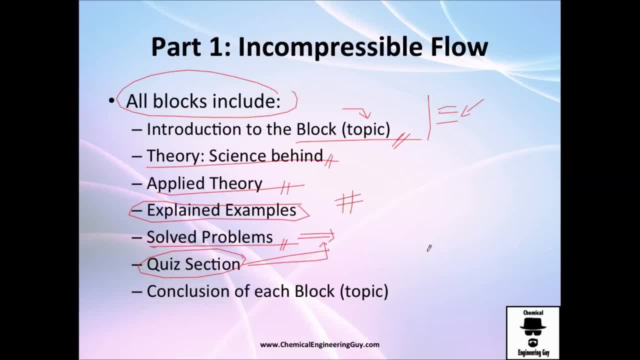 pumps, how to use a pump, what's a pump, what's the pressure, suction cavitation, etc. and of course, each block has its own conclusion. so when you finish the block you don't get the idea that you're just like full of areas we're going to have. the idea of this is to have, for example, what's this? 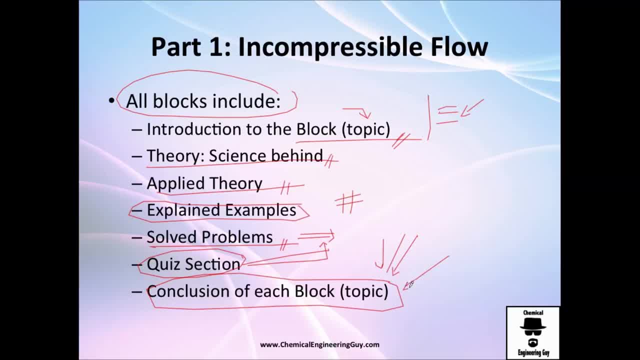 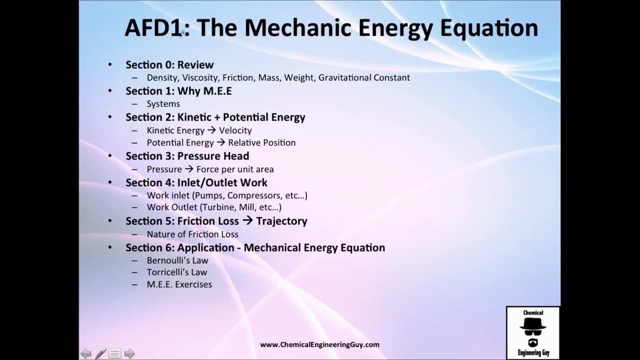 useful for which block is going to need this block? which other blocks are needed or were needed for this? what we? a review of all everything and so on. so let me show you AFD, block number one, the mechanic energy equations. so, as I told you before, section 0 is a review: density, viscosity, friction, blah, blah, very. 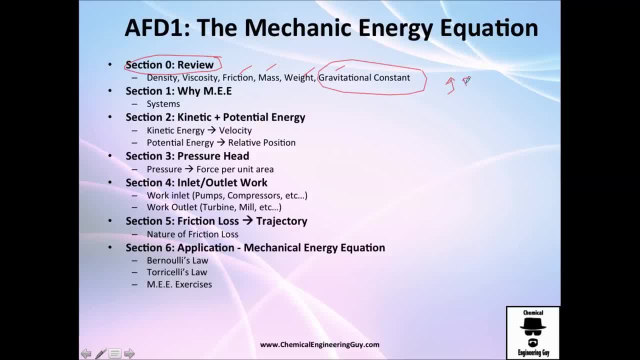 important topic, gravitation constant, which in SI system is number one, beautiful number one, and for English system is 32, as usual. very strange. why do we need the mechanical energy equations for example, systems, how I apply systems, systems? why do we need kinetic and potential energy? you know kinetic is. 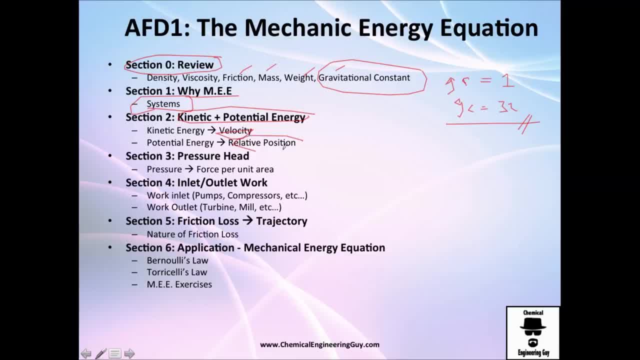 about velocity. something that moves definitely has energy. something that has a very relative position with respect to gravity has also energy. the pressure head, famous pressure head, which is force per unit area and inlet outlet, work- how to calculate or account for pumping, compression turbines and so on. and we 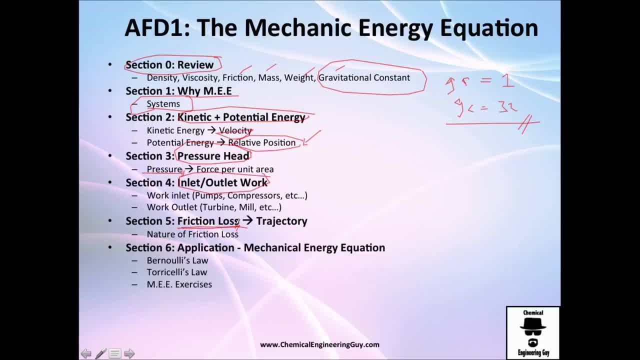 check out a little bit and instead let's say an overview on friction loss. it's a dependent on trajectory and the nature of friction loss. why do we have friction? and finally, we check out some examples. we do the Bernoulli's law example, Torricelli's law example and the complete or full mechanical energy. 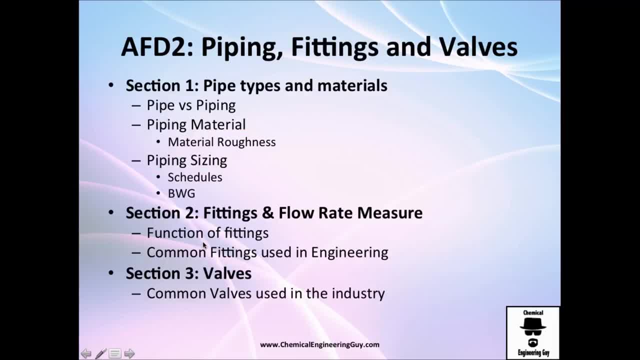 equation examples. so after that will be interesting to check out piping, fittings and valves. we have three sections essentially. section number one is pipes and types of material. what's a pipe, what type of material that we use, roughness of the material and sizing, which is very common in the industry. then we go to fittings. 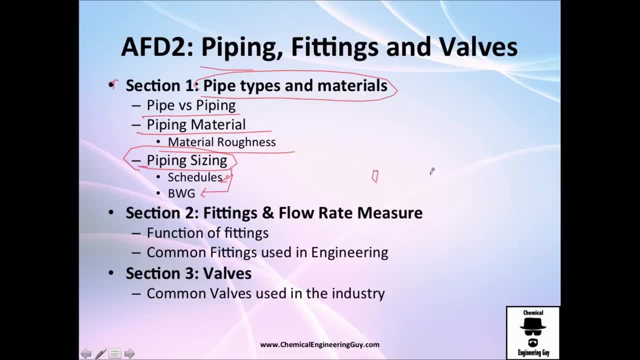 and low measurement, actually stuff that you add or plug into your pipe in order to have a function. for example, you want the valve to control volume, you want a pressure meter calculate pressure differentials, you want a- I don't know an L to change the direction in 90 degrees, and so on. the function of each and many common 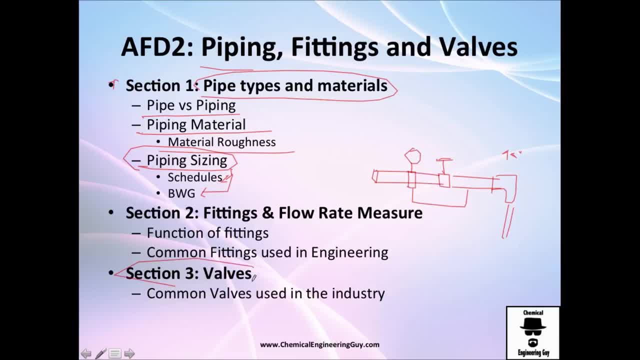 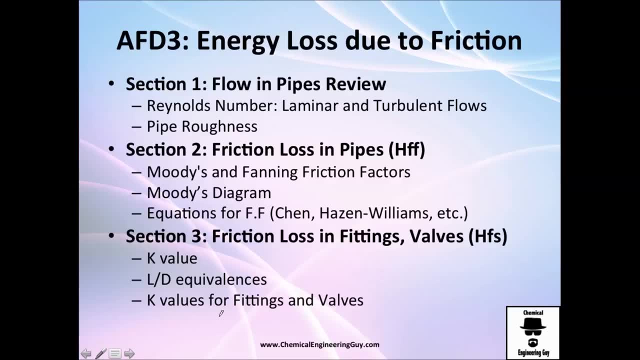 fittings used in engineering. and finally, as I tell you before, valves: common type of valves. and why do we have many types of valves? then we go to AFD, block number three, energy loss due to friction. so we have a little review of flowing pipes, the Reynolds number, laminar flow, turbulent flow. then we check out section 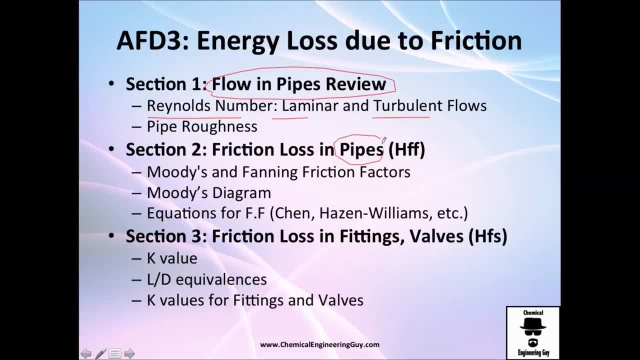 number two, which is friction loss in pipes, because we also have friction loss in fittings on bulbs. of course you know that if you have evolved partially closed, let's say 90% closed, you are going to have a lot of friction there. so we see a little bit on Moody's and fanning frictions or definitions. 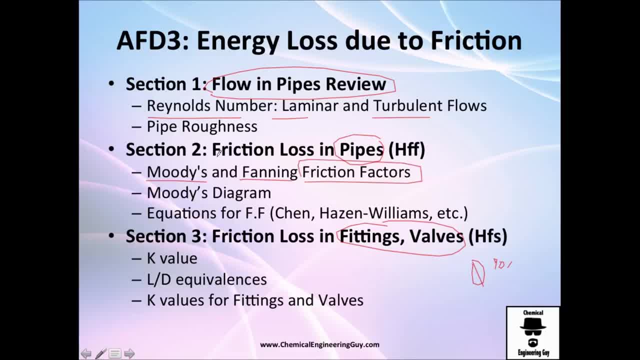 of friction factor, the difference and which one. we will be using the Moody's famous diagram to calculate friction or relate friction factor, friction versus Reynolds number and many equations, because actually it's pretty good to have equations so you can use them on Excel's or spreadsheets or even 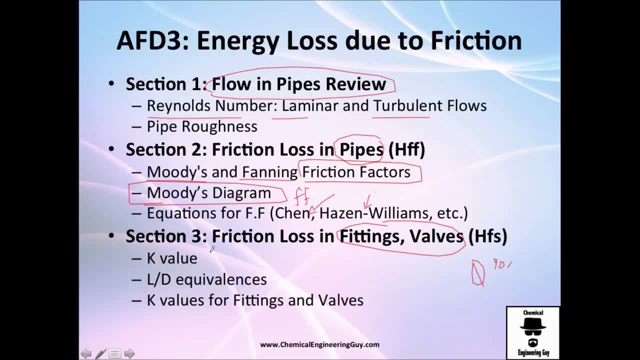 calculators instead of having a diagram. now, once we understand friction loss in pipe or pipe wall, we're going to check out what's the friction loss in that fitting or valve, for example. how do we calculate that? how do we do equivalences? actually, if you were to have this elbow, what's the equivalent on a pipe, for example? 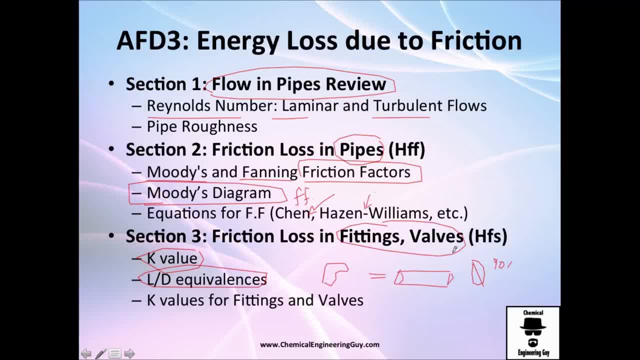 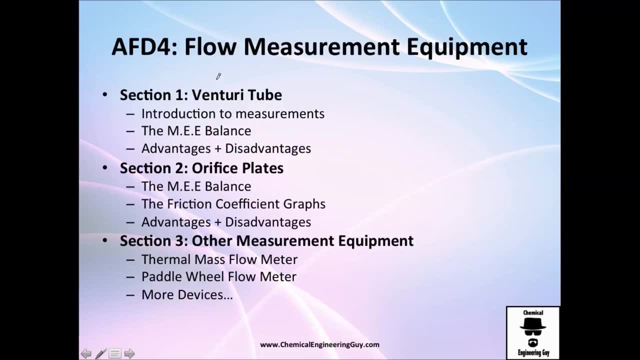 having this elbow will be the equivalent of losing two meters of this pipe, and so on many types and many values of fitting and valves. so I told you before about measurement equipment, so we're going to check this in this aft, block number four, section number one, venturi tube. 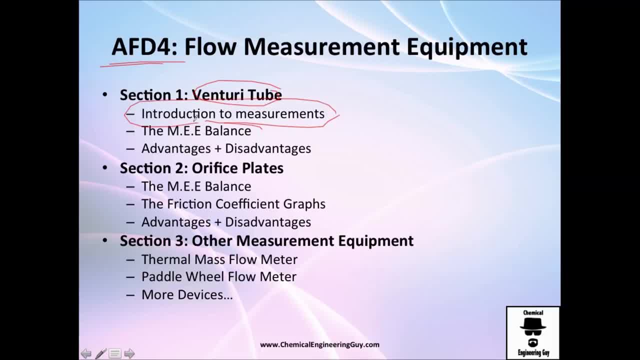 Let's check out introduction and how to do a mechanical energy equation balance and why is it good to have a venturi tube and why is it bad for disadvantages. then we go and check out the artifice plate, which is easy to move and change. this is actually difficult to be changing every time, or if 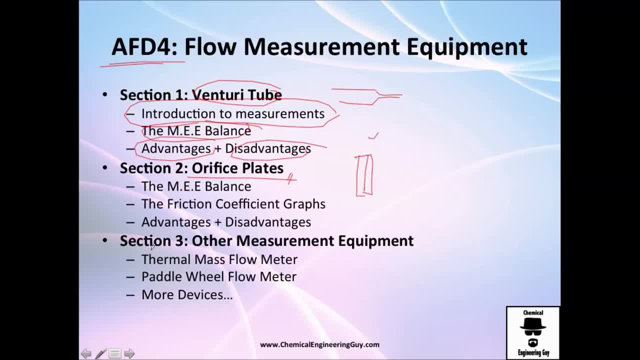 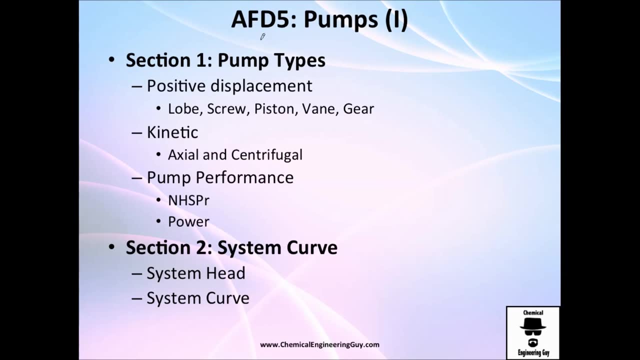 it's plates. it's good, but it's kind of expensive. and finally some state-of-the-art measurement equipment such as thermal mass flow meter, paddle wheel, magnetic and many other devices. So then we check out pumps. AFD, block number 5, this is 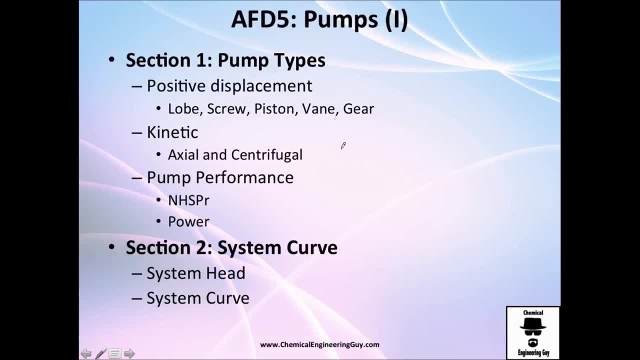 essentially five sections. section number one is theory: what type of pump do we have? positive displacement, kinetic and a little bit on pump performance, such as cavitation and so on. then we check out the system curve. what's the system requirement actually? so if you have A needs to go to B and you calculate the. 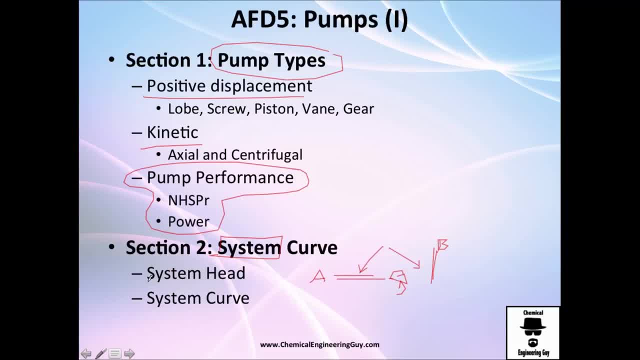 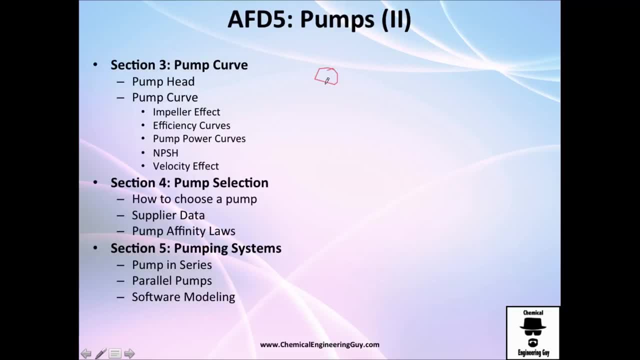 amount of energy required for this system. so this is the system head, and then we will be able to calculate the amount of energy required for this system. so this is the system head, and then we will do a system curve. we will see that later then for different pumps we're 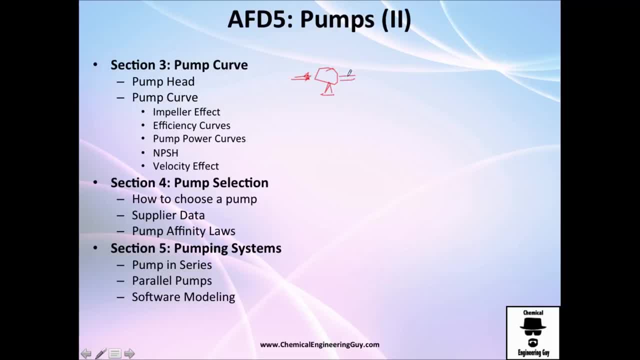 going to study. you make an energy balance here, and an energy balance here only on the pump. that will be the pump head and we will do a pump curve. not only that, we're going to see the impeller effect, the efficiencies curves, the pump power. 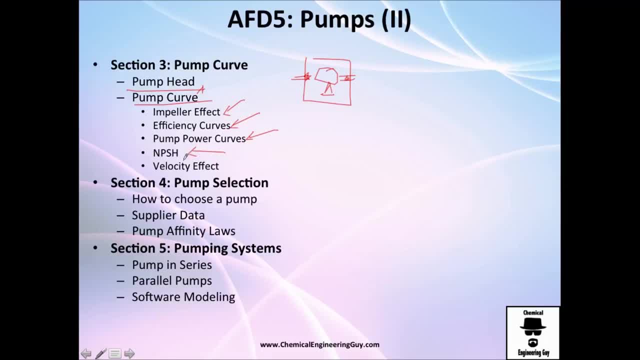 curve the net positive displacement needed and the velocity of the revolution per minute of the pump. so we will see a lot of pump curve here and then finally we can go and see what's the best pump to choose, how to choose a pump supplier. 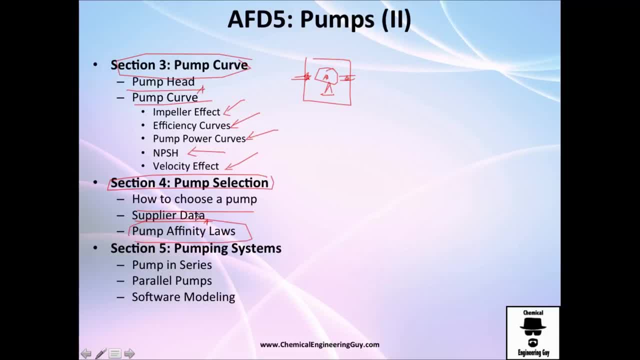 data commonly added and affinity loss, because many times we're going to have a diagram which is not complete, but with these rules, with this loss, we will be able to calculate a point away not included in our diagram. so, for example, Then, pumping systems, pumping series, parallel pumps and software or common software used to model pipes and pumping systems. 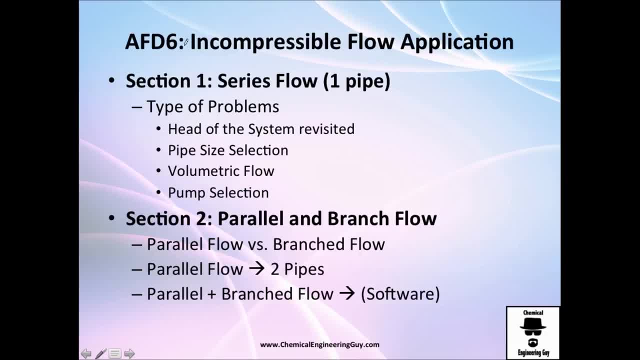 We are almost done, guys. once you know all the theory behind how to calculate work friction loss, pressure loss and so on, We are going to check out applications, real life problems, For example series flow. you have series flow is pretty common, for example here here. 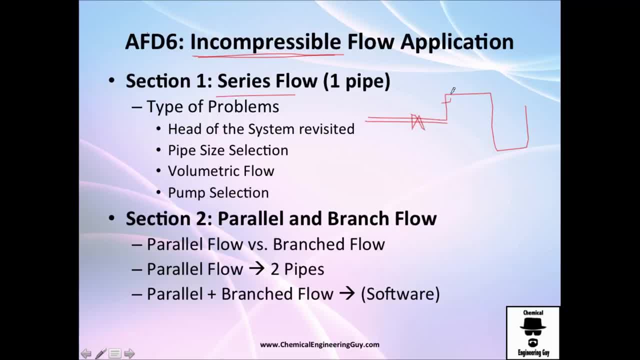 You have, I don't know, maybe valve here and elbow here And you have. this is, for example, 3 inches pipe And this is a 2 inches pipe. And if you have- I don't know, maybe you here- you have a pump and so on. 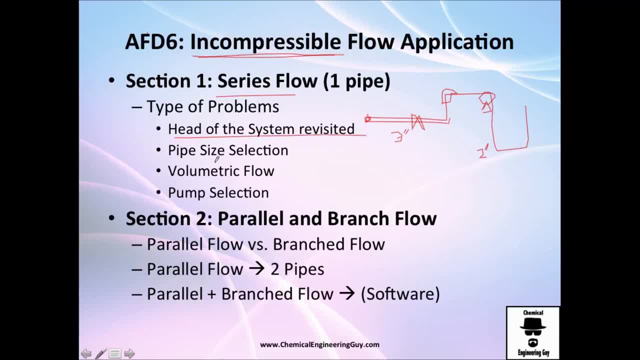 How to calculate the head of the system, How to calculate the best pipe size That you have, The diameter for this system, And even how to calculate the volumetric flow rate that best suits this problem. And finally, some pump selections. That was for series flow. 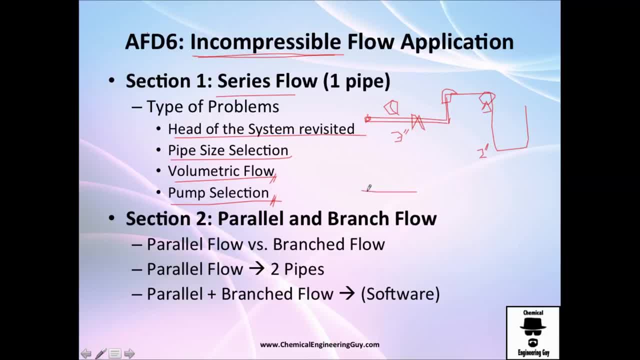 For parallel and branch flow is a very other approach. For example, this is pretty common in the industry You have here, it goes out and then meets once again in another place. This is parallel flow. Branch flow is a very, A very interesting concept. 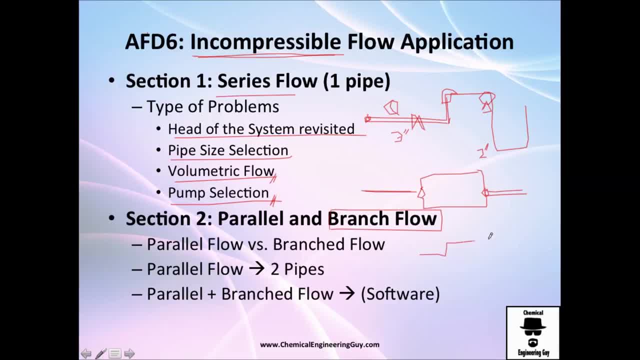 It's actually more difficult and complex to model. For example, you have this point right here and then this one goes right here And this branches once again, And the thing here is that the flow meets again here in parallel flow, Let's say with two pipes. 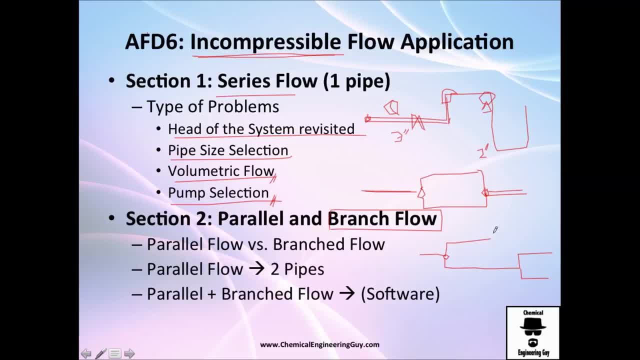 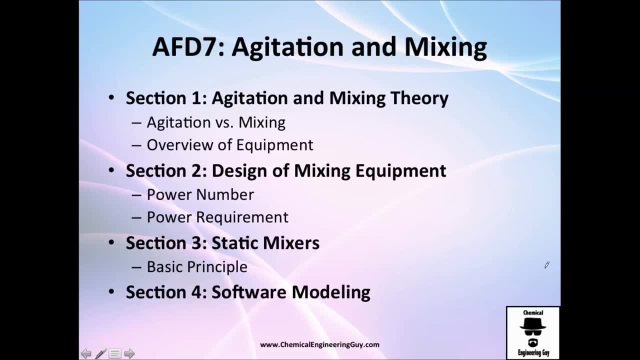 And in parallel or branch flow. with more than two pipes, for example, they never meet. So it's very difficult to calculate this. You will need to use software. And finally but not least, we check a little bit on agitation and mixing. 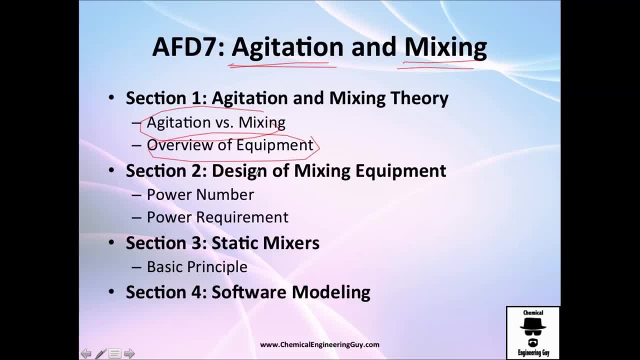 The difference overview of equipment. Then we start to actually design the equipment, For example, power number and power requirement. Then we go and check out this very fancy stuff which is static mixers And some software to model that We're not going to see how to model it. 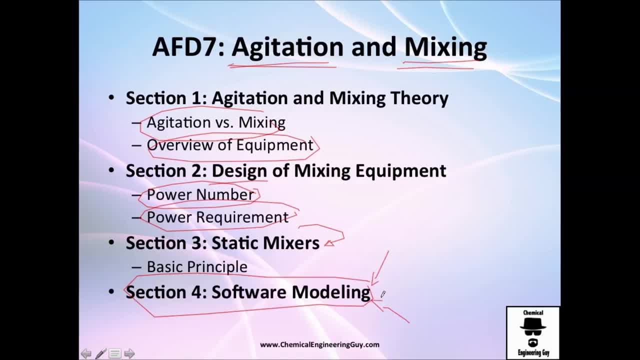 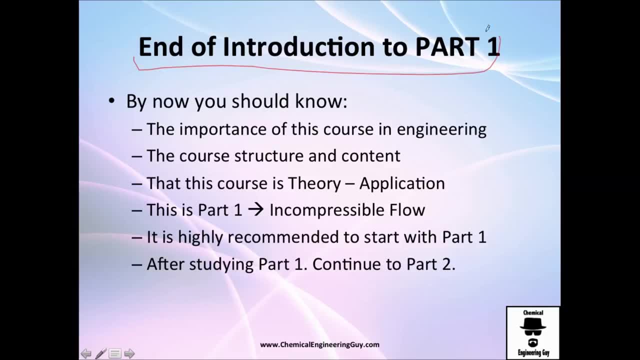 Just the software that exists to model that. We're going to see how it works. We're going to see how it operates And, thanks God, we're done. This was the end of the introduction of part number one, which is incompressible flow. 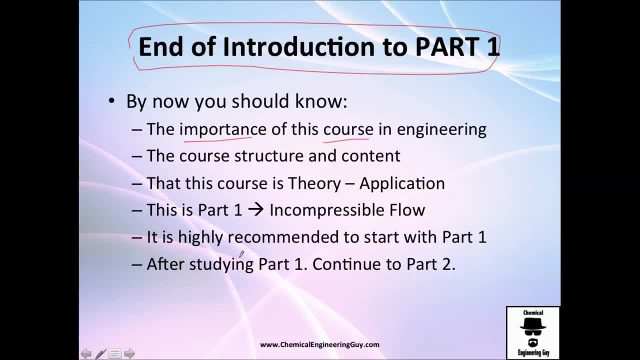 By now you should know the importance of this course, The course structure and content, That this is a course of theory but mainly application And, of course, hopefully you know by now that part number one is incompressible flow liquids And I will definitely recommend you guys to start with part number one. 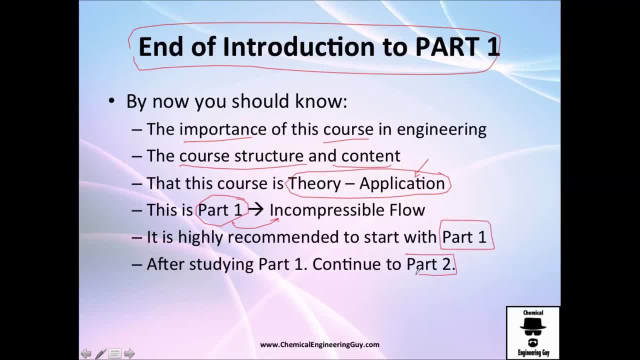 You can, of course, go directly to part number two, But you study part number one, you will get more easy part number two And I will definitely recommend you guys, If you're done with part number one, go directly and study part number two. 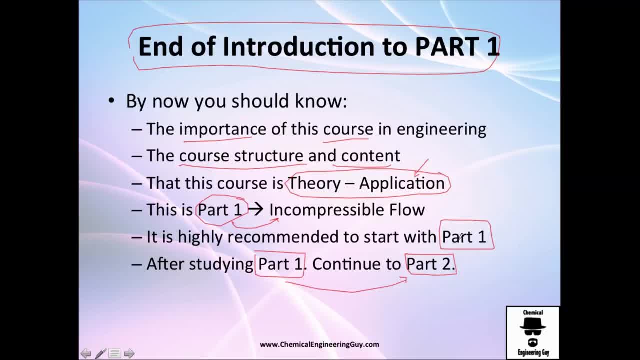 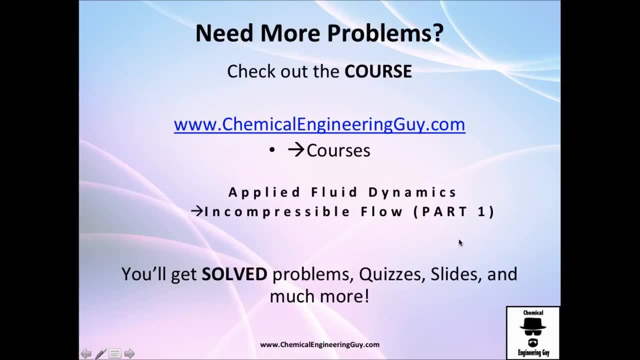 Once that you are fresh, then you can get it everything, Because if you let time pass then you will not remember part number one And part number two will be a little bit more tricky for you. And, of course, guys, I have a lot of problems for you. 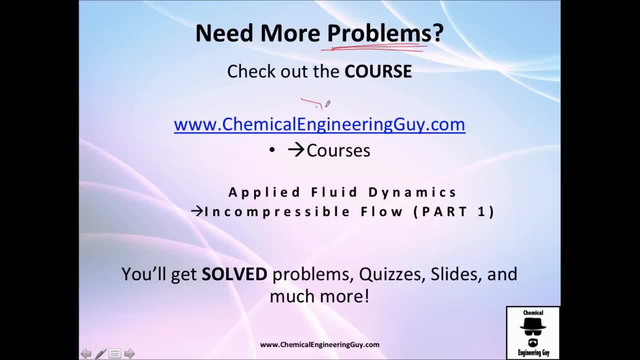 This is exercises on solving problems. Go and check it out. Go to chemicalengineeringguidecom courses, Choose applied fluid dynamics, Go to part number one, which is incompressible flow, And you will get a lot of solving problems, quizzes, these slideshows and much more stuff.